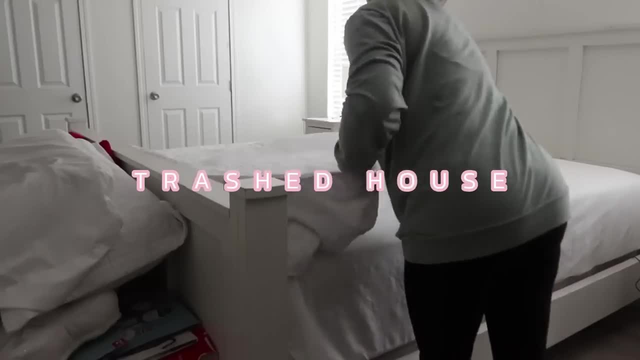 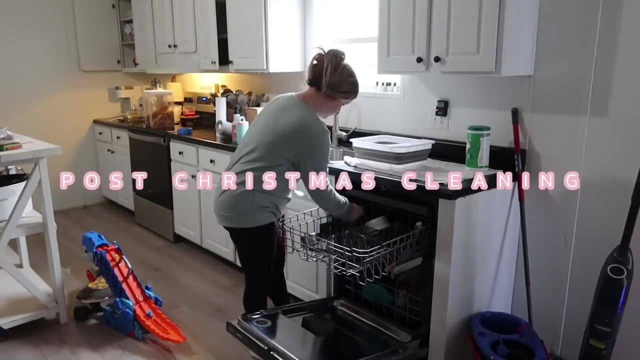 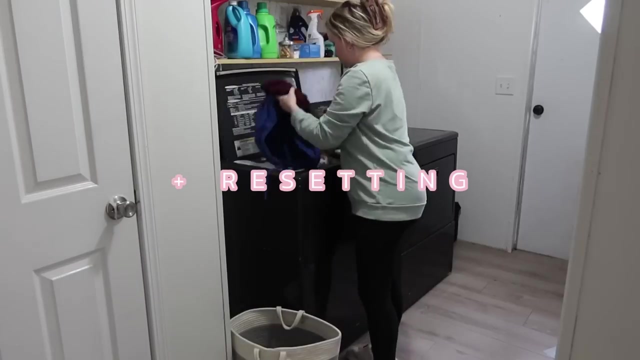 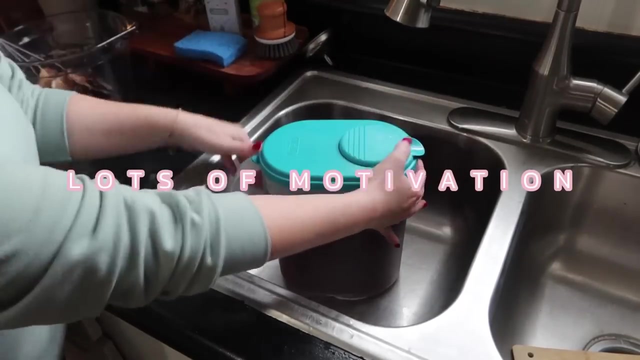 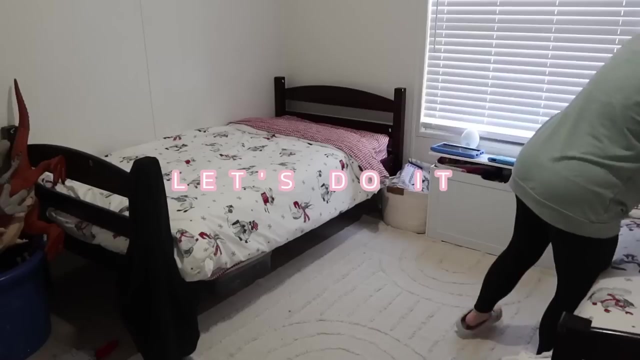 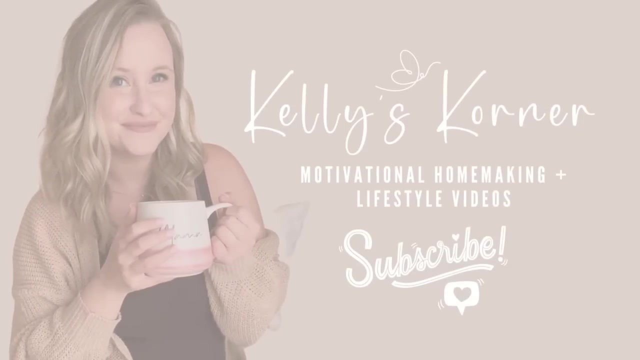 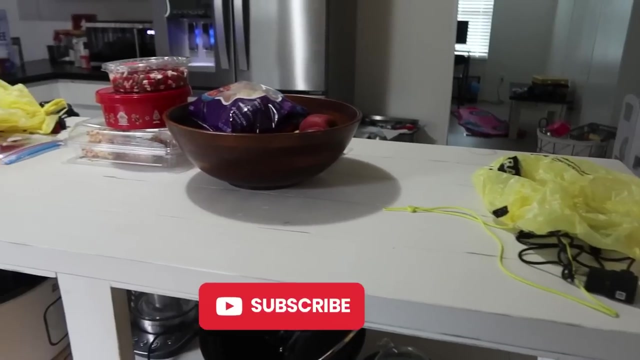 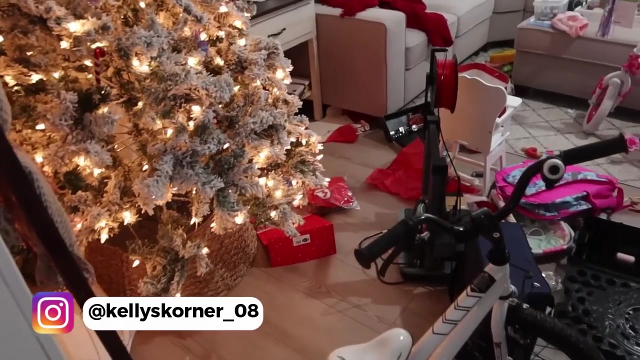 Thank you for watching. Hey y'all, and welcome back to my channel. Today's video is an after Christmas clean with me. My house was totally trashed after Christmas morning and I didn't do a lot of cleaning on Christmas day because I really just wanted to spend time with my family. We also had somewhere that we had to go. 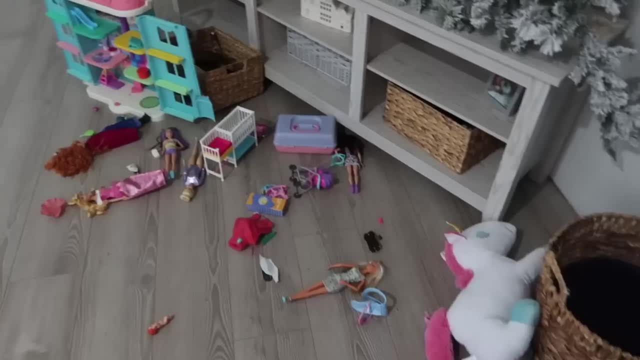 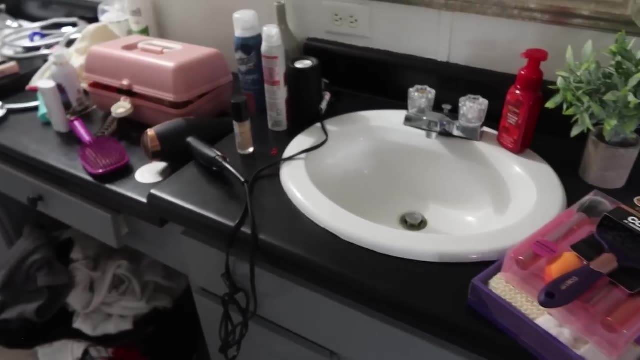 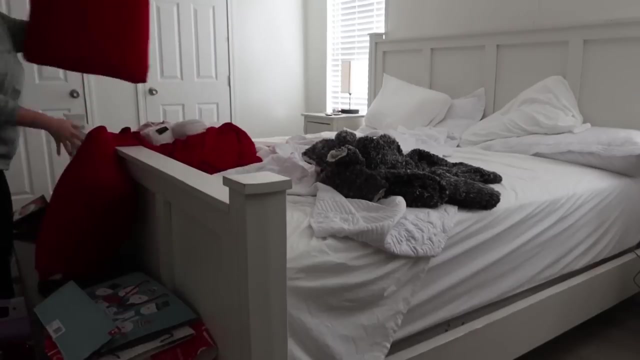 and so I just kind of left the mess and enjoyed the day. So the day after Christmas I got busy getting my house in order and I decided to film it for you guys and give you some motivation. if your house is like mine and completely trashed, I hope this video will give you the motivation to get it back in. 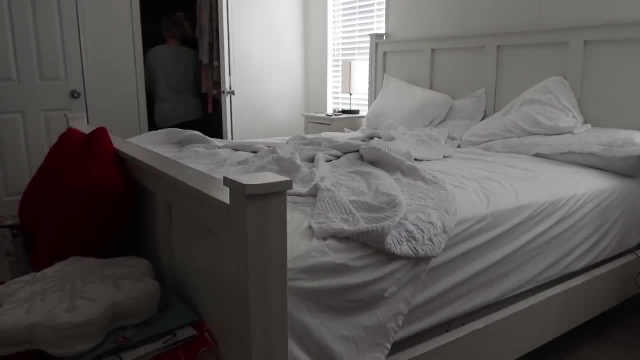 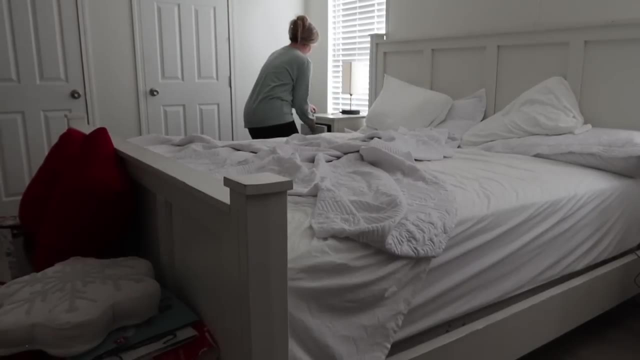 order. I'm not trying to get my house perfect today. I'm just trying to get it where it's not so chaotic. So I had about three or four loads of laundry that I had to fold, and so what I did is I'm going to make my bed up and then I'm just going to throw the laundry. 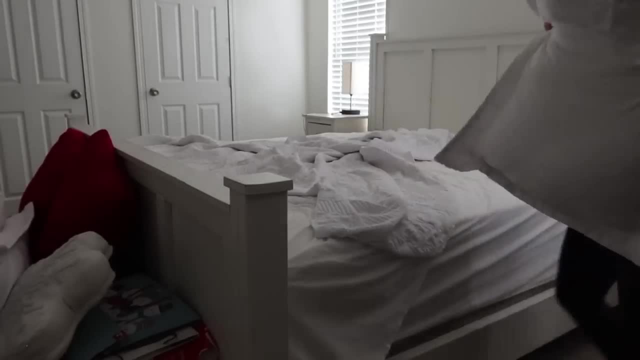 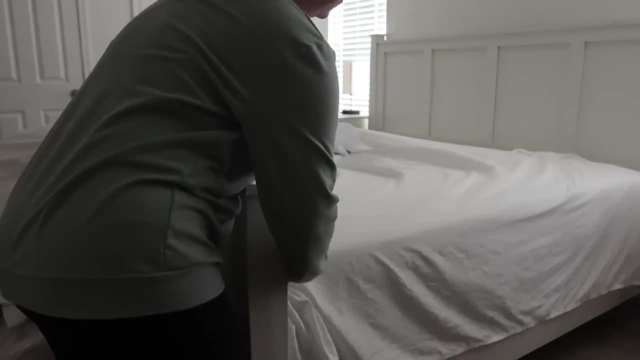 onto the bed. I'm not going to get it folded today, but I'll at least have it all in one place and hopefully tomorrow can get that folded. So that's the plans for the laundry. but yeah, I hope you guys had a wonderful and merry Christmas with your family. We had a really good Christmas. The kids. 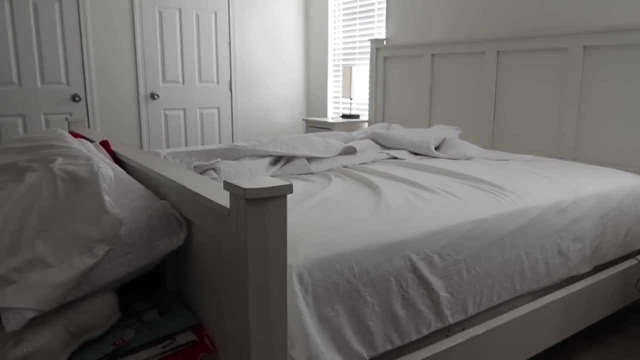 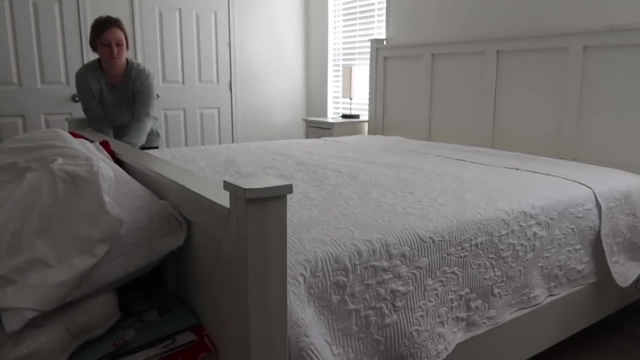 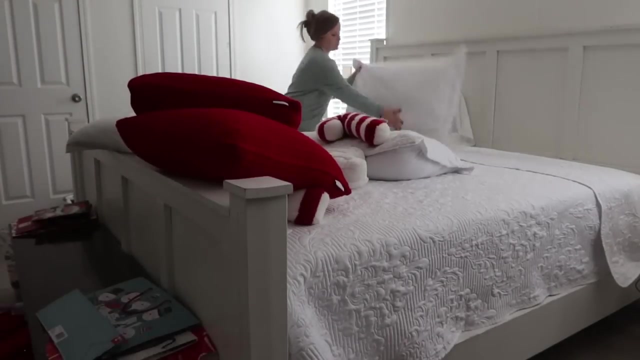 were so happy on Christmas morning opening up all of their gifts, and it was just so much fun watching them. I swear when I was a kid I thought that I would be disappointed to grow up and have to spend Christmas as an adult, but as it turns out, it's actually so much more fun to be an adult and make the magic happen. 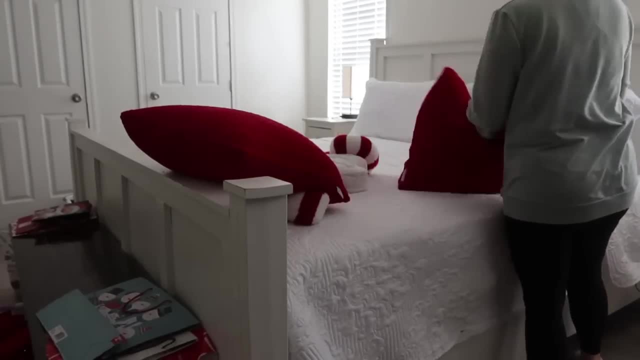 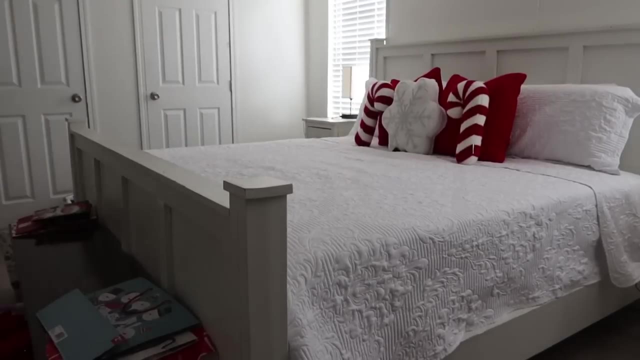 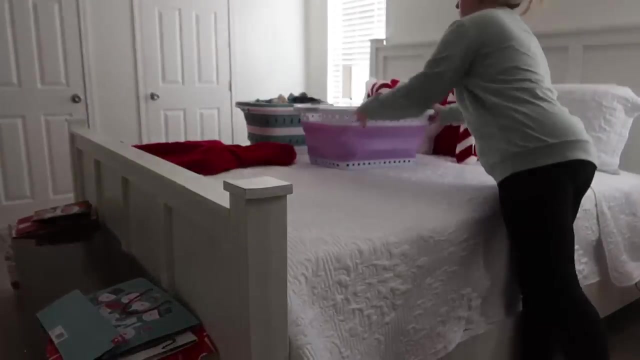 for your kids. But now that the fun is over, I've got to get this house back in order. It was complete chaos. I had a really hard time going to bed last night with my house in complete chaos, but I was so exhausted by the time we had finished with Christmas morning and all of our Christmas. 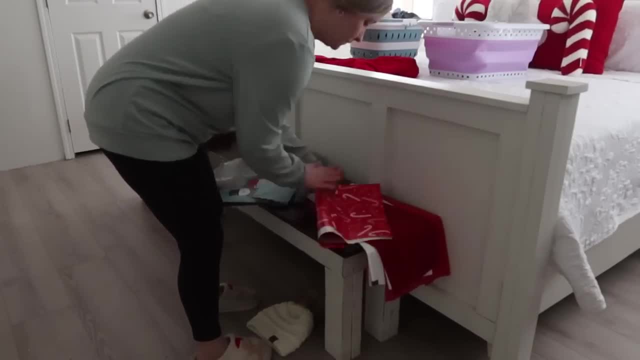 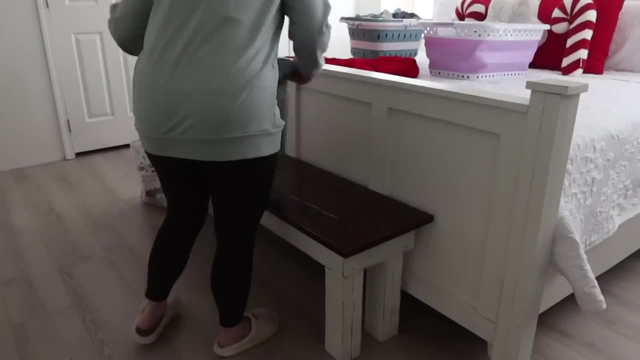 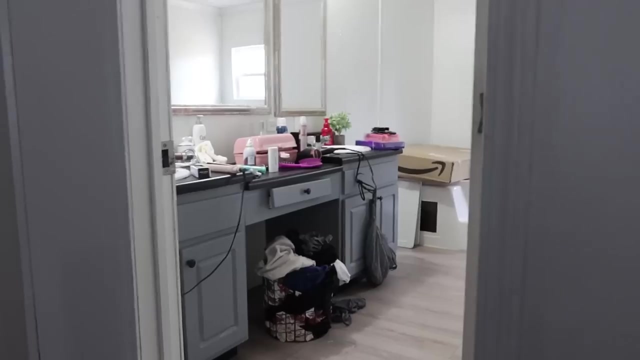 activities that we had going on that day that there was just no way that I could get it cleaned up. So I went to bed with my house a mess and when I got up this morning I was a little overwhelmed. so I decided I would just go room by room. So I'm starting at one end of the house. I'm going to get 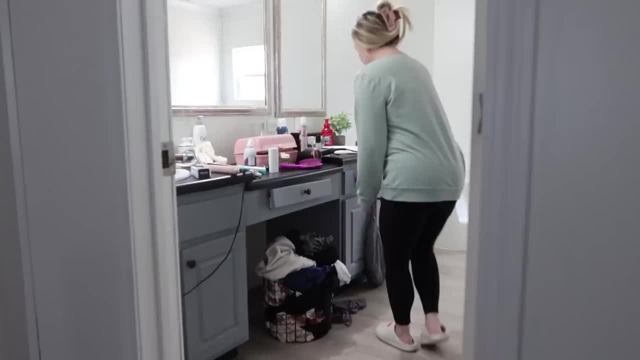 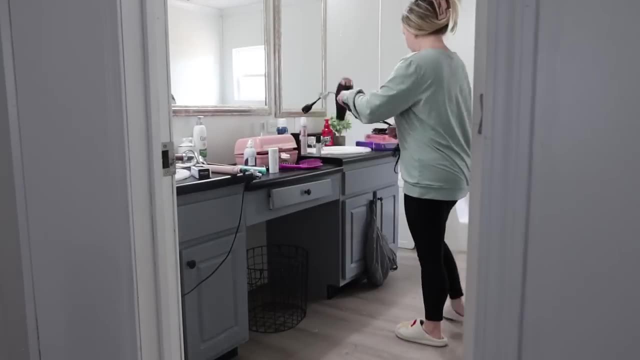 my bedroom and my bathroom straightened up and then I'm just going to work my way down. But all throughout the video I'm going to play some upbeat, motivating music. So if you have some cleaning to do, pop me up on your TV and let's get it done. 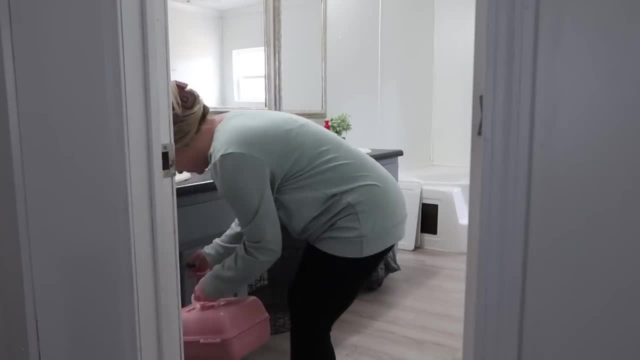 uit. I'm going to turn it off so that I can go to bed. I'm going to leave my house, take over the AC and then fill the computer with the water. I'm going to take a short break and then I'm going to go to bed. 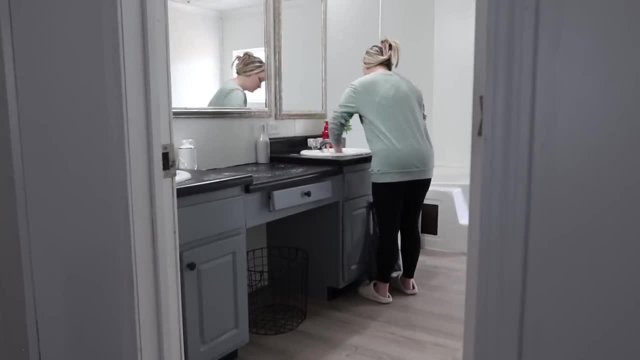 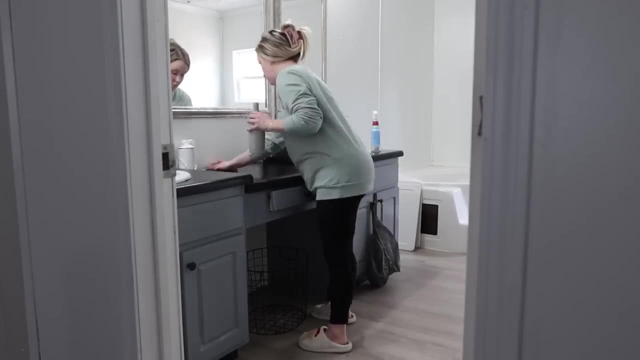 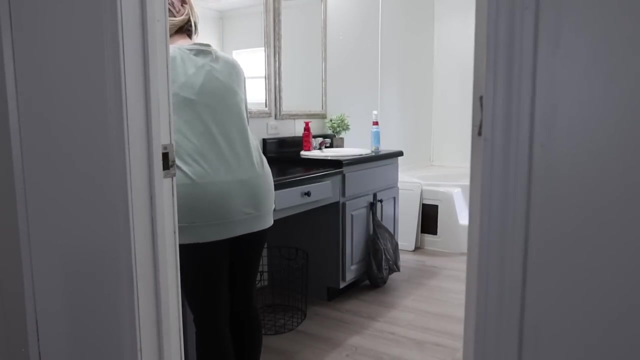 So I'm just going to hang out for a couple of hours and I'm going to ride on my bike and then I'm going to go to bed, I'm going to wake up and I'm going to go home. It's a great time for me to be in that car. I just want to dance. 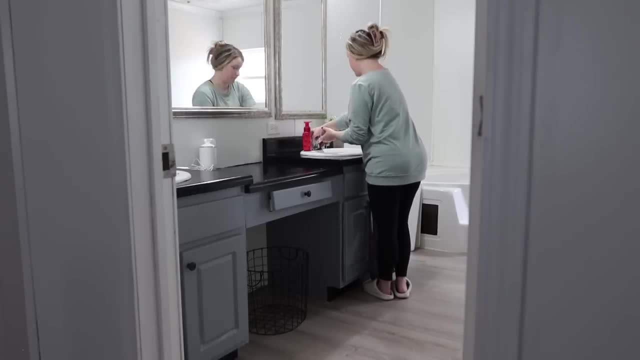 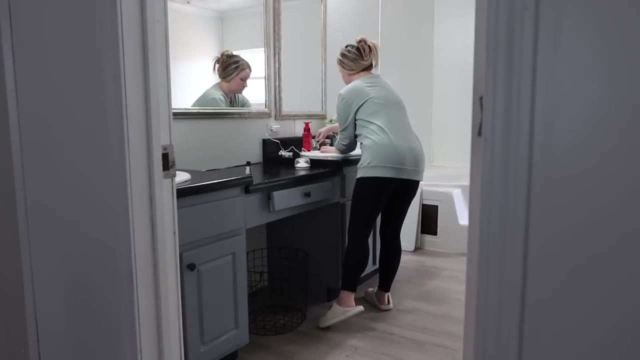 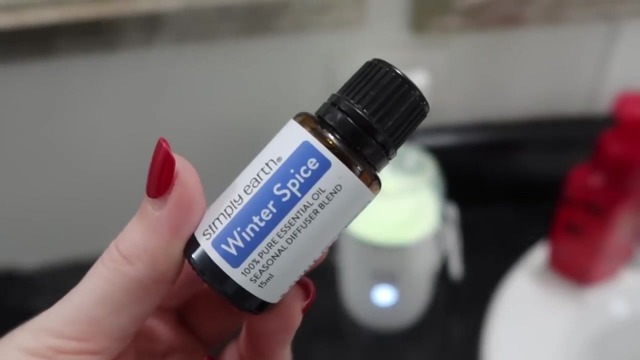 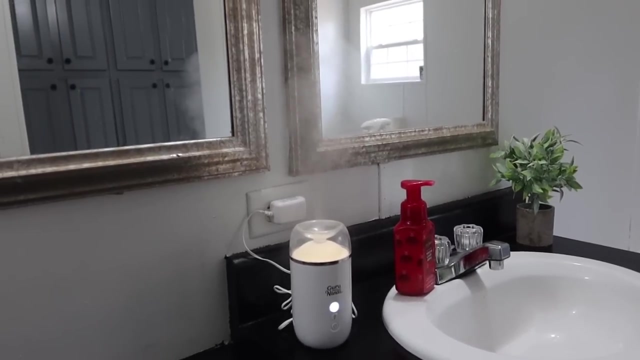 I just wanna dance till my heart goes la-la-la. I just wanna dance. It ain't about money, it ain't about the coolest job. It's about having fun and love the ones that make you shine And you. it's all about you, No matter what the others say. 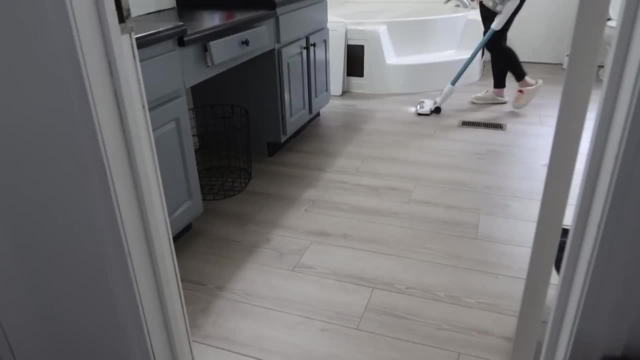 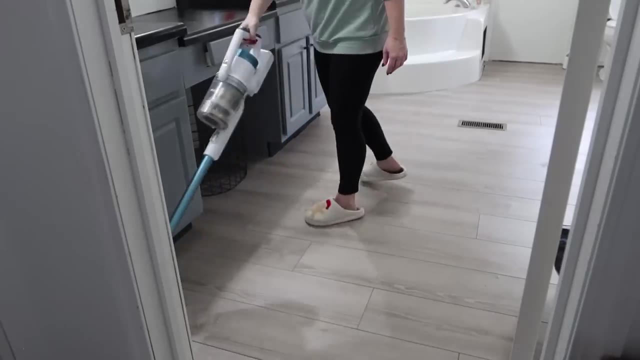 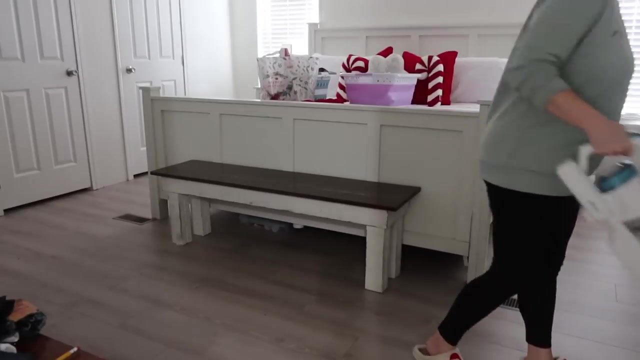 But now I'm done talking the lights on me. I tell you, I guarantee this. That's why I take a turn for the better. Now the rain is pouring and all I see is Lightning around my feet. Now nothing can bring me down. I just wanna dance till my heart goes. la-la-la. 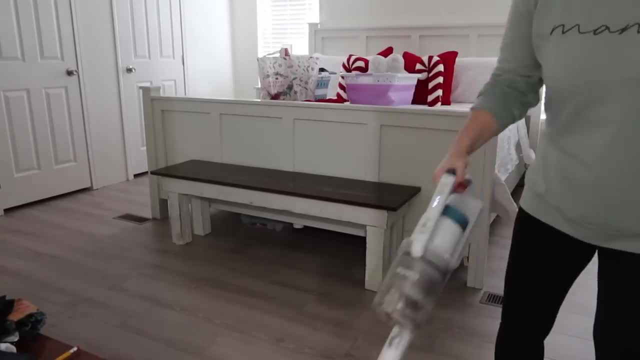 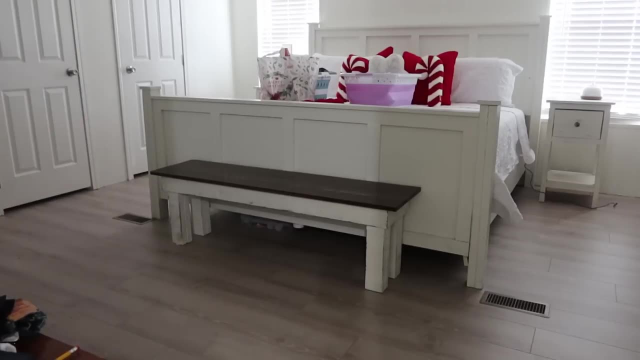 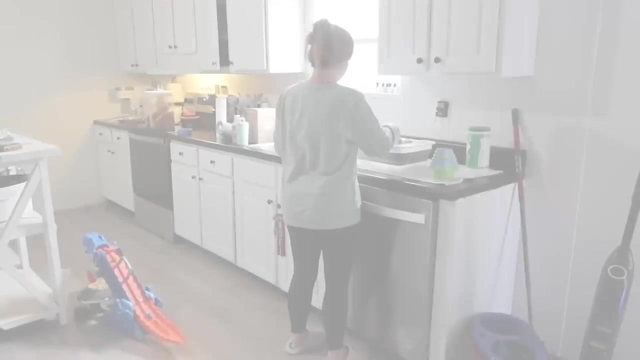 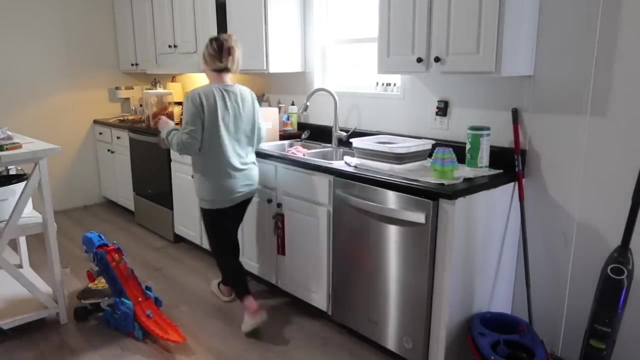 I just wanna dance. I just wanna dance till my heart goes la-la-la. I just wanna dance. Moving into the kitchen, I'm gonna go ahead and get this dishwasher unloaded So I can reload it with dirty dishes. I didn't have a pile of dishes. That's one thing that I did stay on top of through everything. 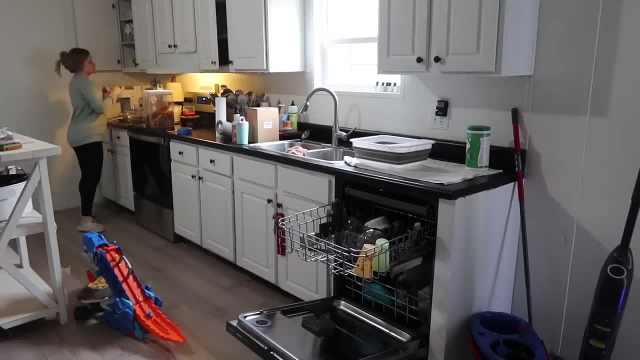 I made sure to keep my dishwasher going as needed, So the dishes aren't terrible, But I do have some new bowls that I got for Christmas. You see those sitting there by the sink. So I'm gonna get those taken out of the box Into the dishwasher, Into the dishwasher. 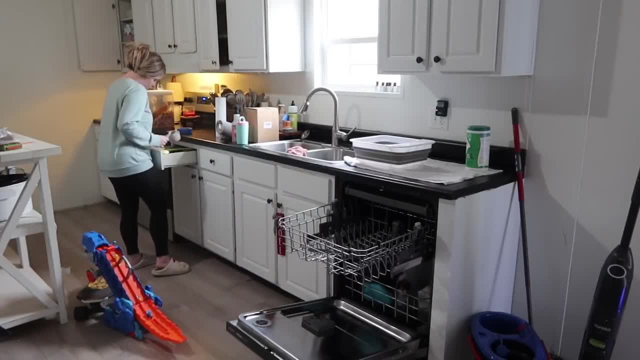 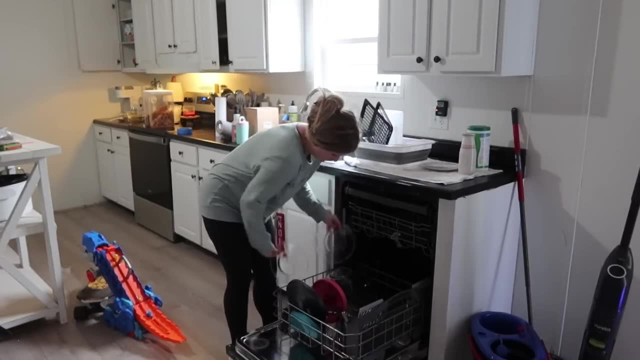 Into the dishwasher And later on tonight I'll run a cycle. We didn't really have enough dishes right now To go ahead and run the dishwasher, So I'm just gonna load what I do have And just get this kitchen cleaned up. I also wanted to scrub my stove top. 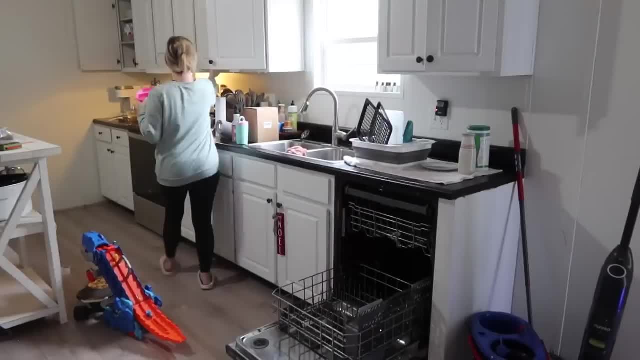 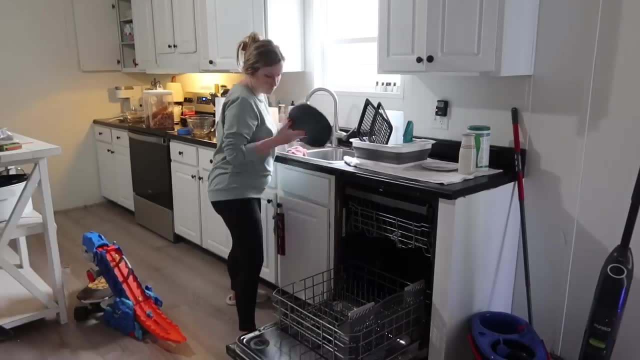 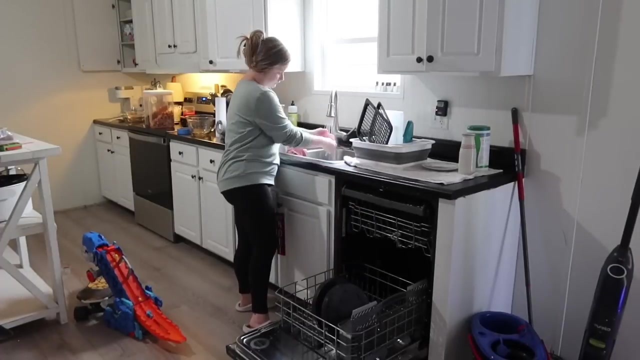 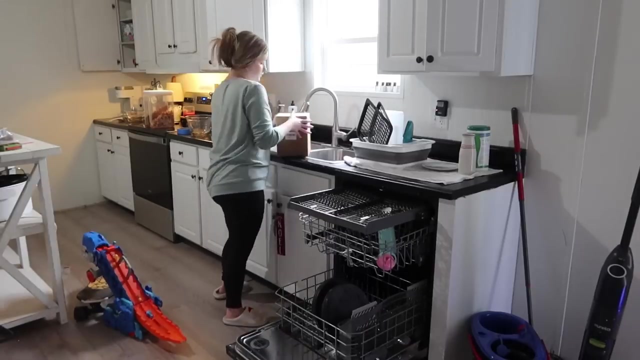 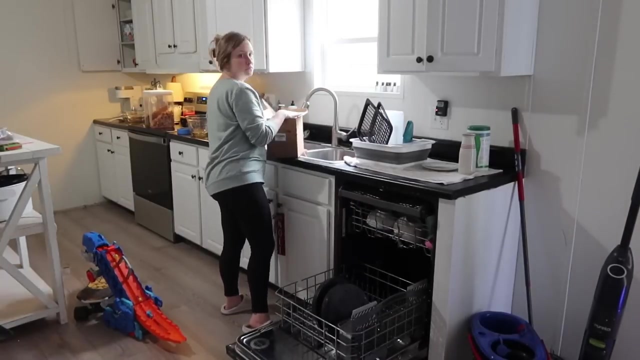 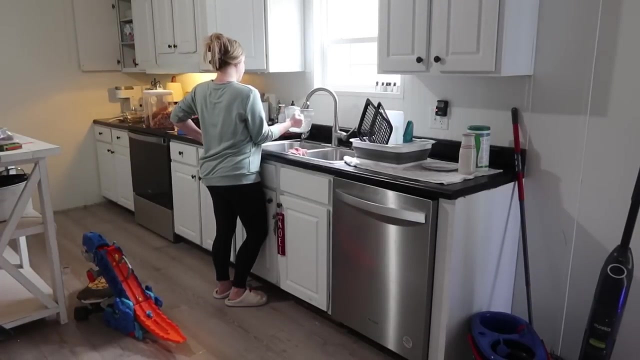 With some Barkeepers brand Scrub out my sink, Wipe down my appliances- All of that. There was fingerprints all over my refrigerator, So I wanted to get that cleaned And shine back up. I'm gonna get some sweet tea on to go in. Sometimes we'll do it on the stove. 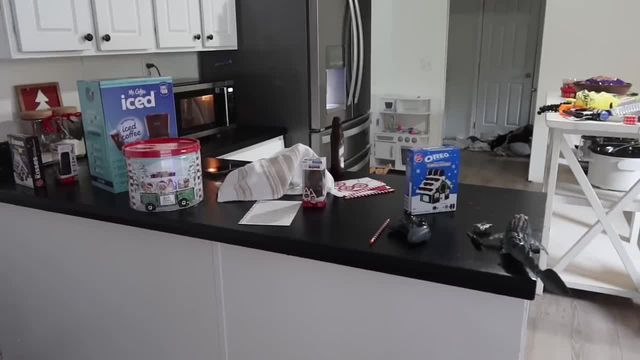 Sometimes I'll do it in the kitchen, Sometimes I'll do it in the kitchen, Sometimes I'll do it in the microwave. It really just depends on my mood. The microwave does seem a lot faster, So I'm gonna get that going really quick And I'm just gonna let it go. 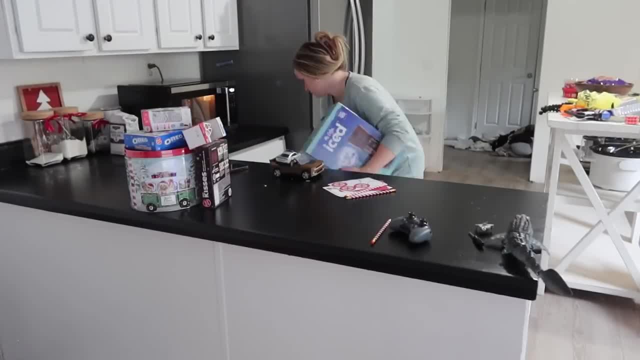 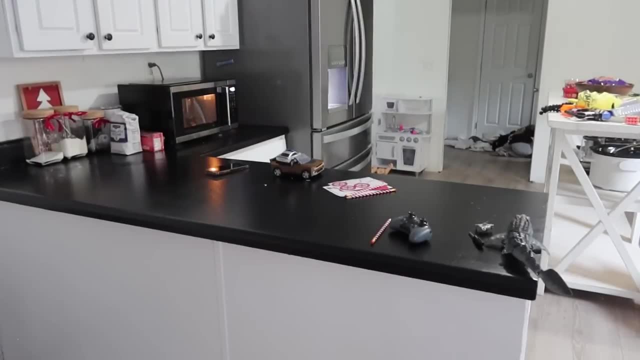 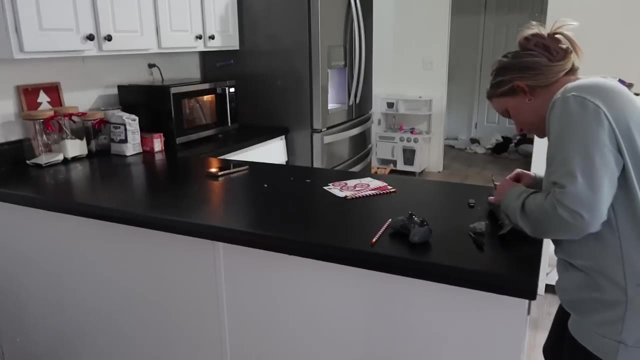 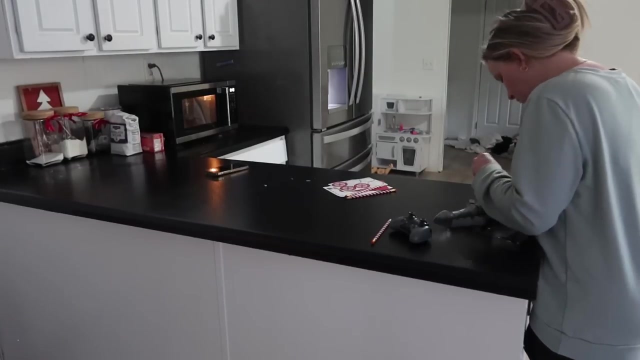 I'm gonna set it for about six minutes And then I'm gonna let it sit for a little while And just steep. So I'll just let that sit While I get everything else done, And then I'll mix it up For about an hour Or so. I'm gonna let it sit for a little longer. 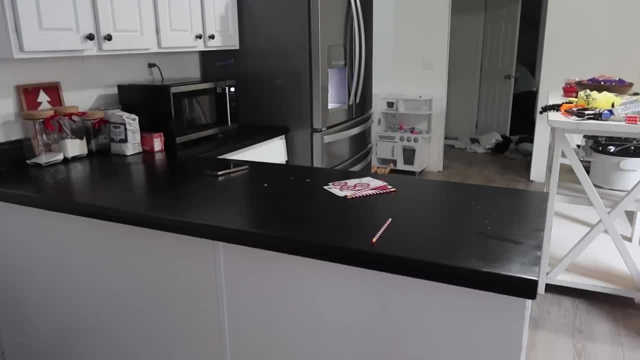 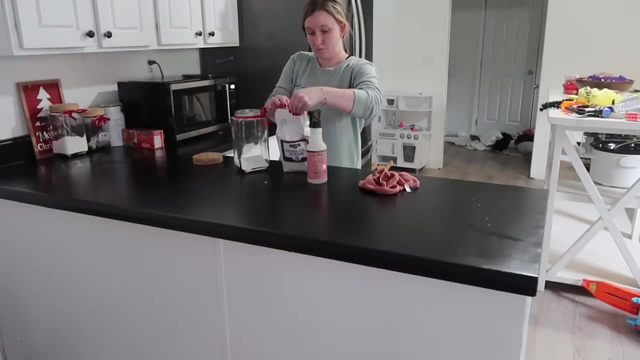 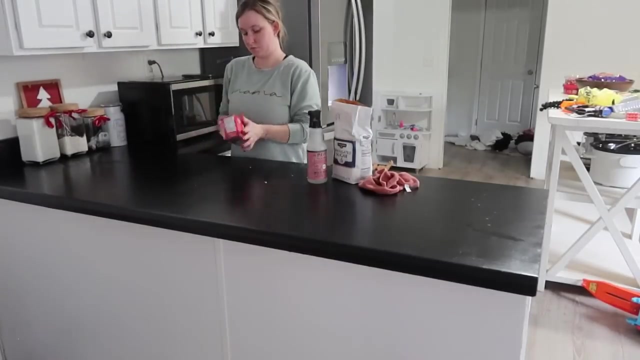 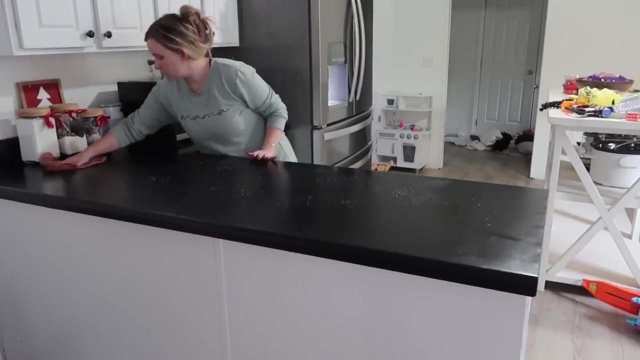 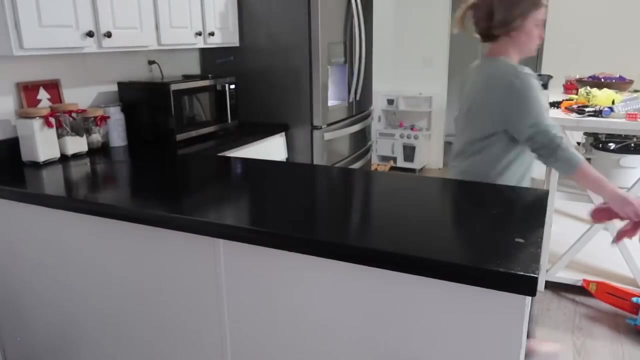 And maybe I'll start the Anybody Pidence It once I've finished, But luckily it took it out Only seconds. Shake the, literally. She's like: come on, i'll have to tell me if there's anybody else out there that's feeling like this, but i am. 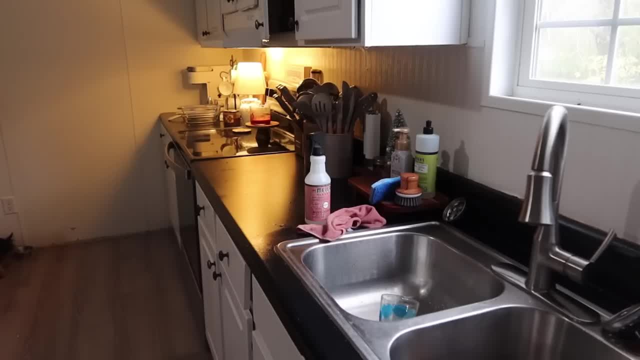 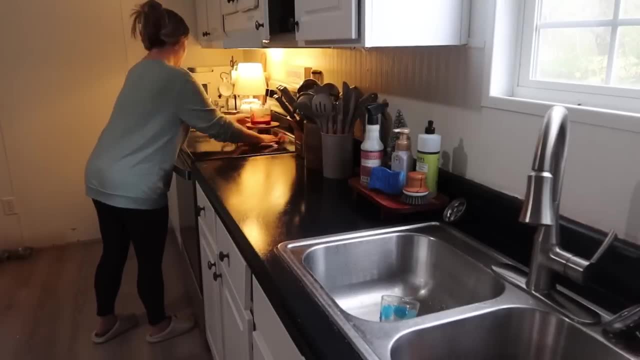 kind of sad that christmas is over. i don't want to take down my decorations, and usually after christmas i'm ready to go ahead and take my stuff down. i'm usually taking my decorations down pretty fast, but this year i just i don't want to take them down. i don't know if 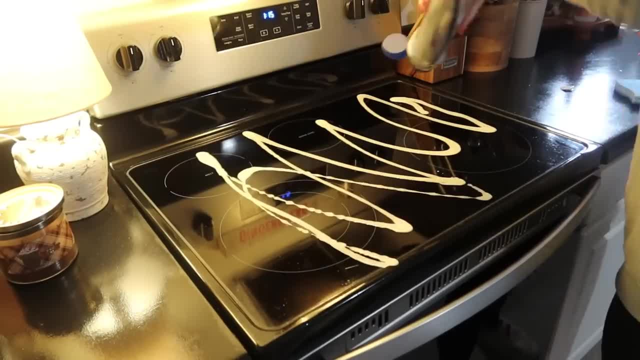 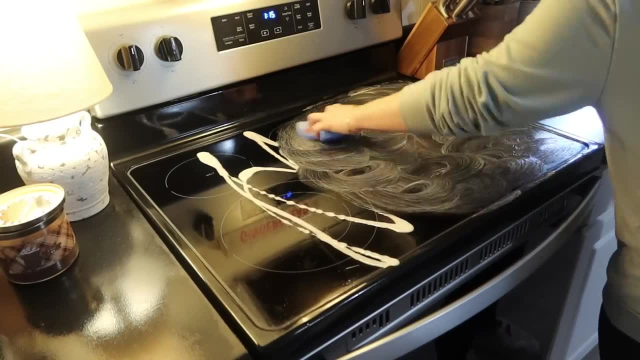 it's because we're in our new house and it's just got everything feeling cozy and i don't know. there's just something about christmas this year that has felt extra special and i just really don't want to take my decorations down, but i think what i'm gonna do is just keep up like my. 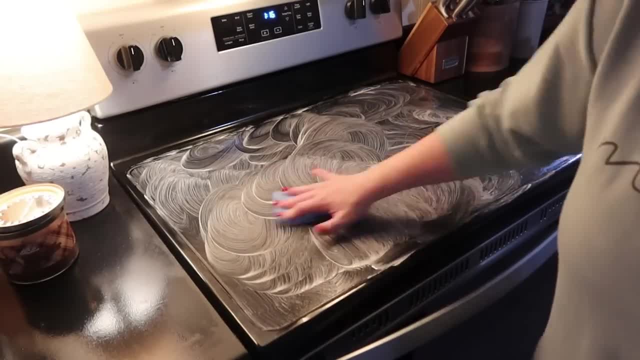 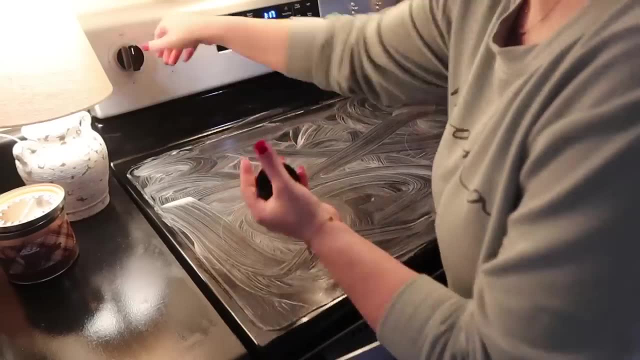 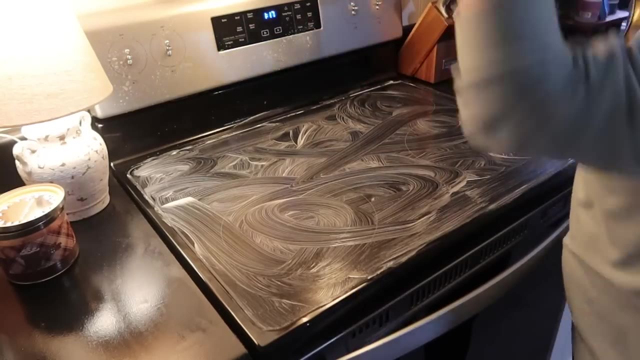 wintry type of decor, so i'm just gonna be taking down anything that's red or that screams christmas. i'll take that down, but i'm thinking really hard about leaving my christmas tree up all through january. i'm gonna be rearranging my living room soon and i don't know how that's gonna work, so i'm just gonna wait until i get that done. 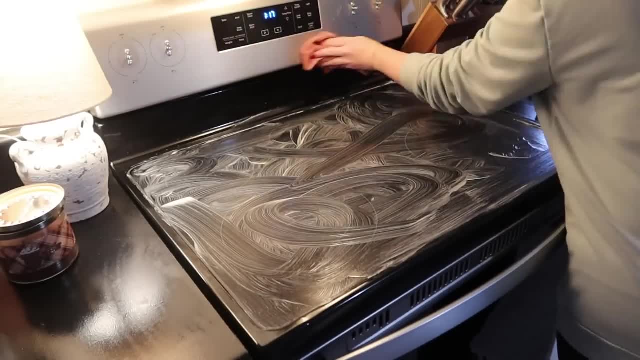 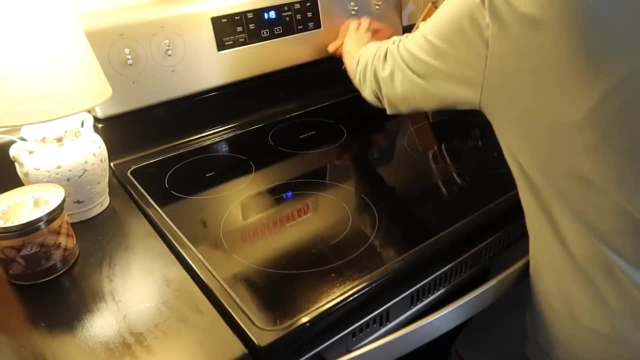 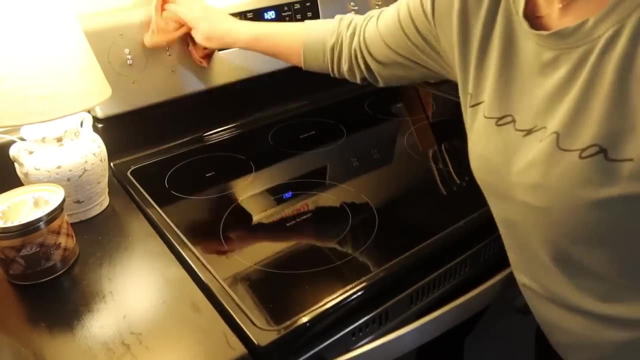 before i officially decide if i'm gonna take it down or not. but i am gonna leave up my wintry decor and just take down anything that's red, so that way we still have all the cozy vibes here in the house. so y'all will have to tell me if you're feeling the same or if you are ready to take your. 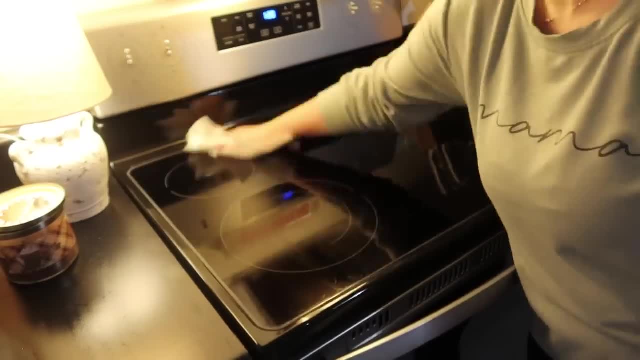 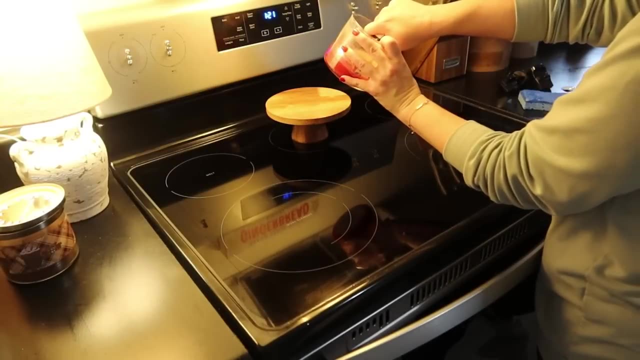 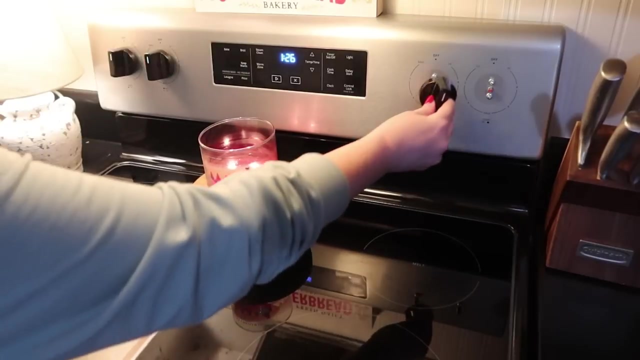 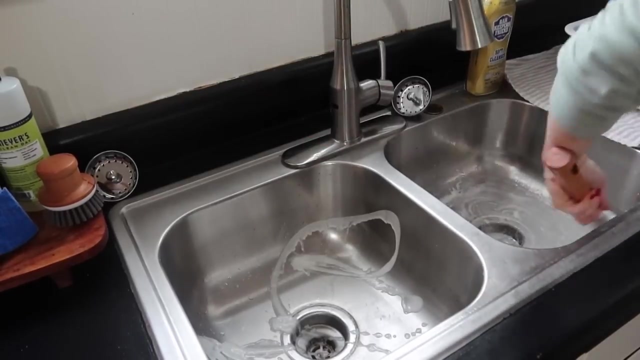 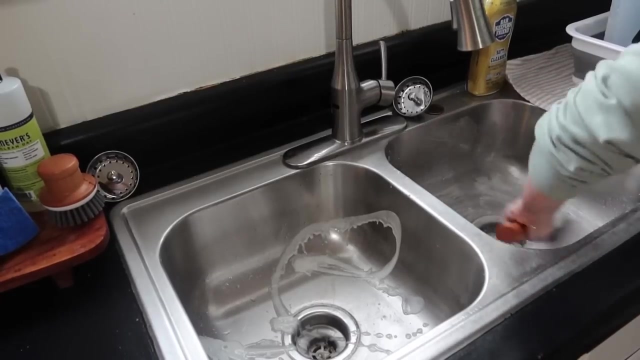 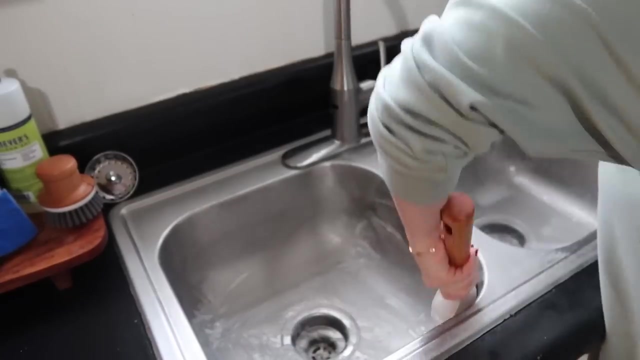 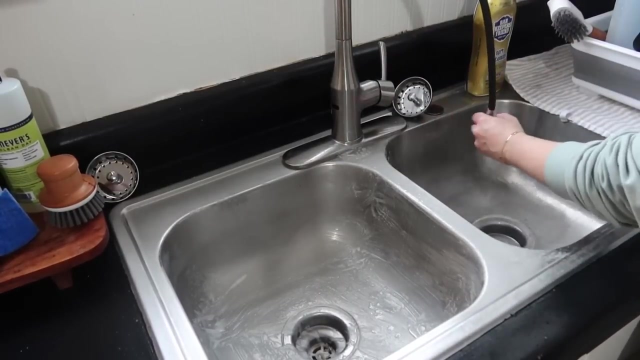 decorations down and i'll see you in the next video. bye, let me know in the comments below i'm staying in this moment, though it's hard sometimes, but i work it out every once in a while. i feel the love. i feel it growing. every day i feel the love. 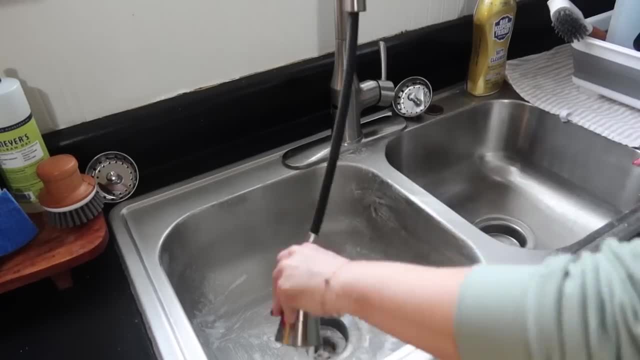 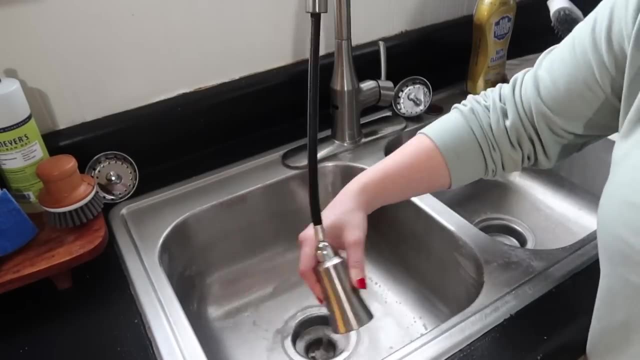 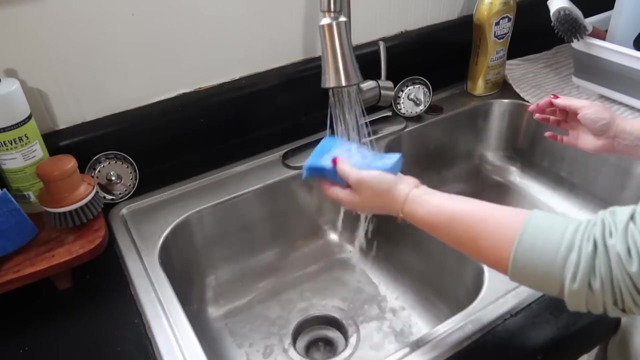 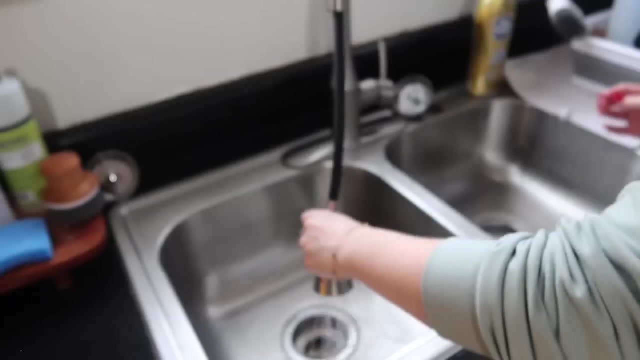 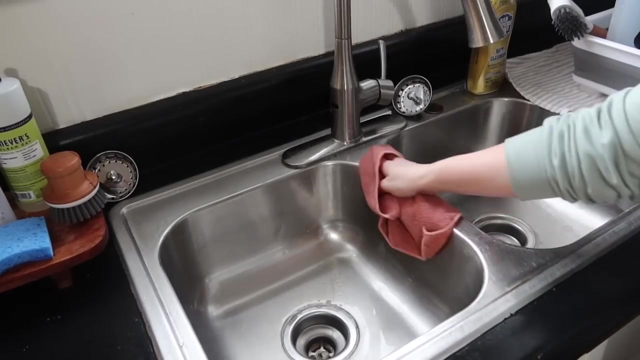 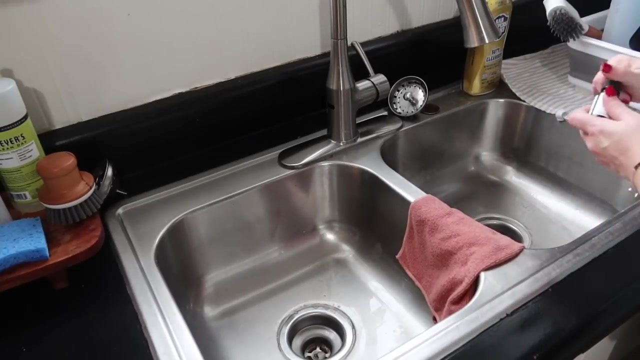 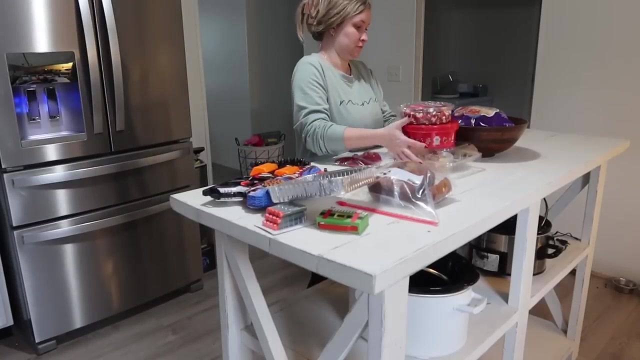 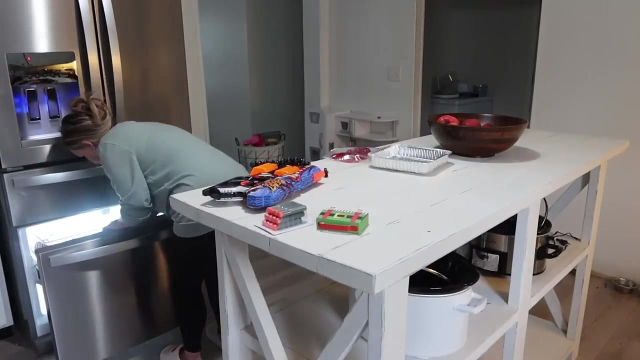 i feel the love. i hope it never goes away. y'all my kids got so much candy for Christmas I don't even know what to do with it all, but for now I'm just putting it in my pantry. There's no way they're gonna be able to eat all of that candy, so I don't know. 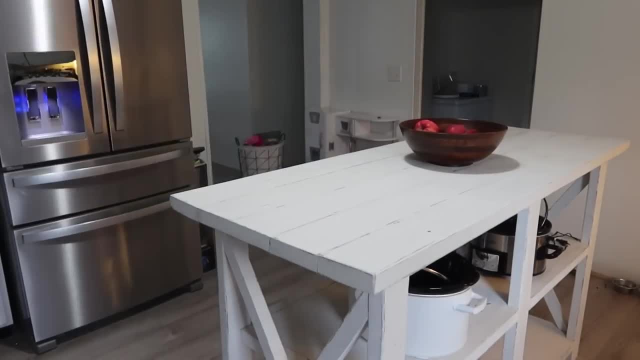 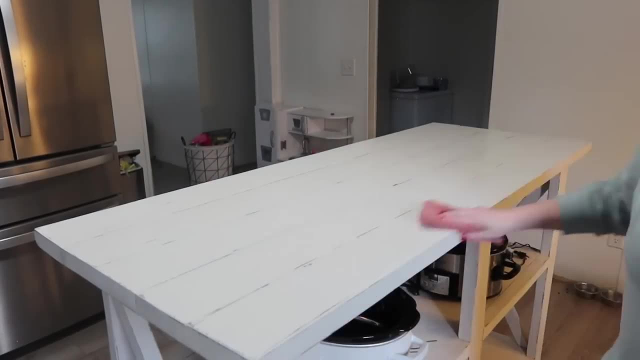 what to do with it, but I'm just putting it up for now and I'll figure it out later. They did get a bunch of Hershey Kisses and I love the peanut butter blossom cookies so I might use those for that, but everything else I don't know what I'm gonna do with. They went to four different places. 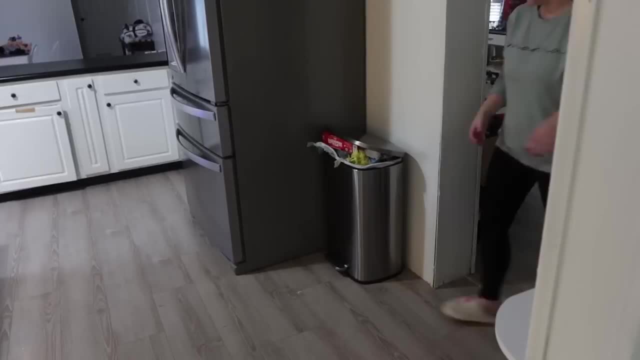 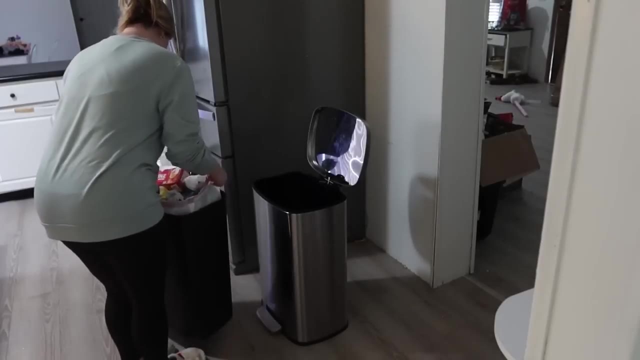 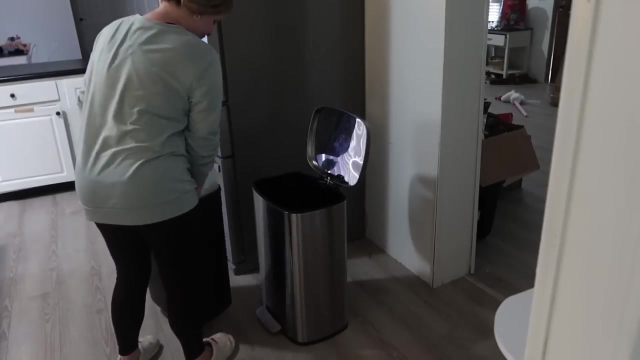 and they got candy from every single place, so we have an overabundance of candy. The next thing I'm gonna do is go ahead and get this trash taken out. We had crab legs at one of our family members houses for Christmas and the kids had brought some home and they had been eating them and then putting. 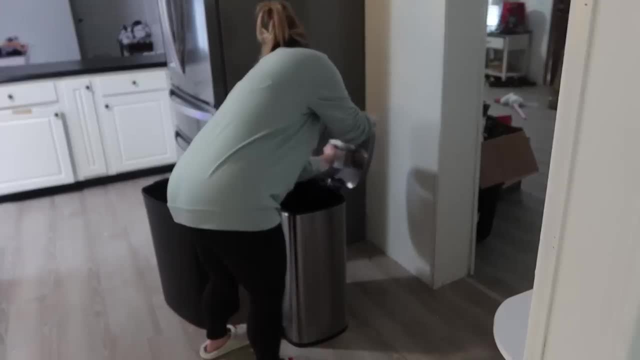 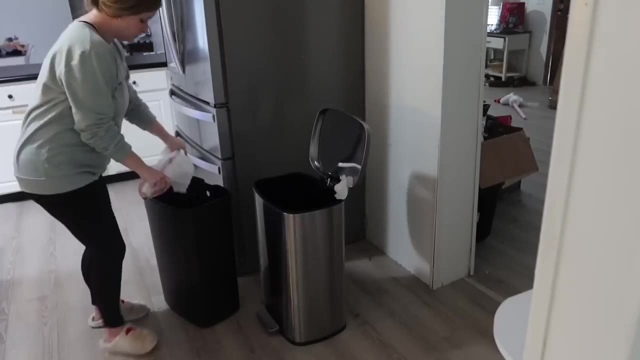 the shells in the trash and I could smell just a little hint of crab. so I'm gonna go ahead and get that taken out and wipe down the lid of the trash can as well. It was kind of cruddy. I'm also gonna take my sprayway. 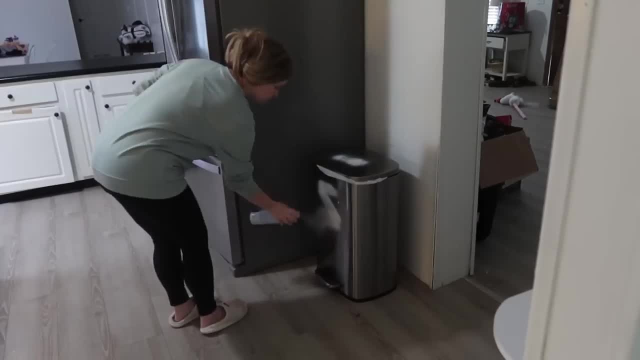 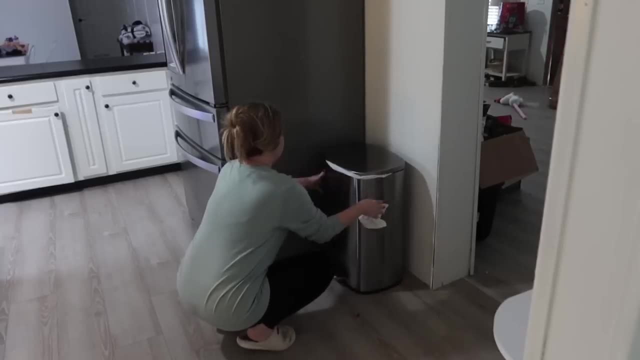 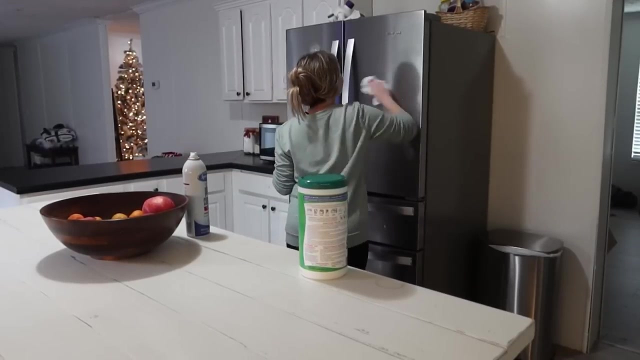 Glass cleaner and just wipe the outside of that really good. I love to use sprayway on my stainless steel. I had found out accidentally that it works on stainless steel. I was using the Wyman's stainless steel cleaner at one time and I had reached for it in my cleaning cabinet. 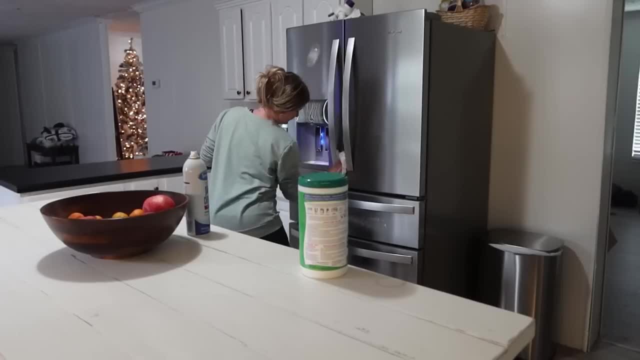 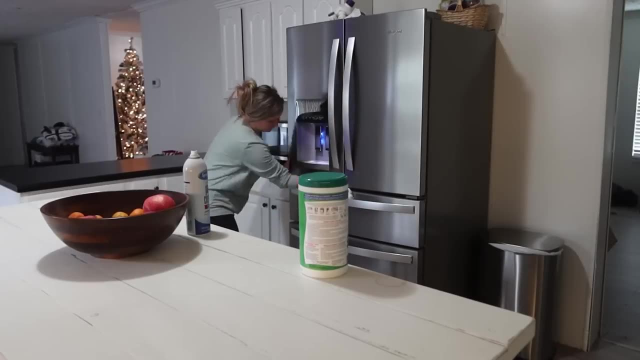 and had accidentally grabbed the sprayway and had used it before I realized and it actually worked really good. so that's what I've been using lately: is the sprayway, glass cleaner on all of my stainless steel and it works really well. Life goes up and it goes down. 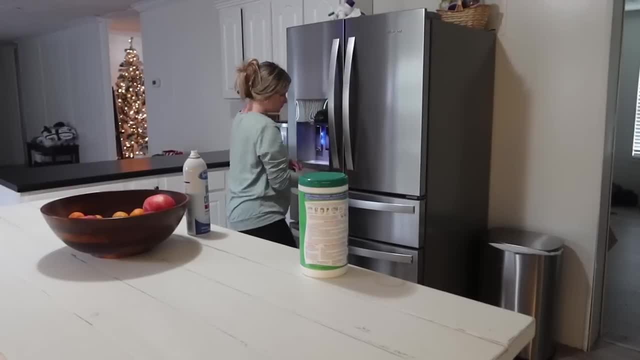 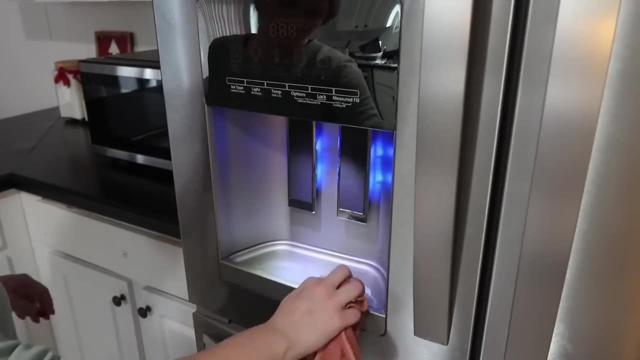 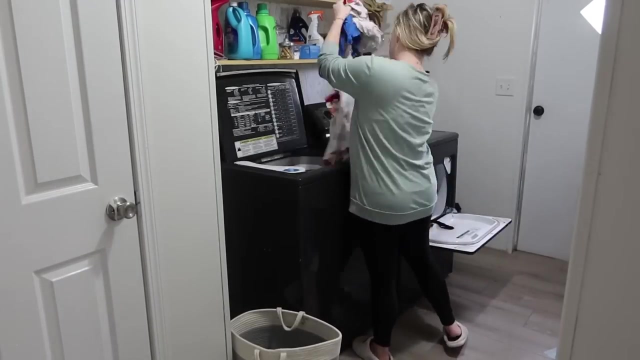 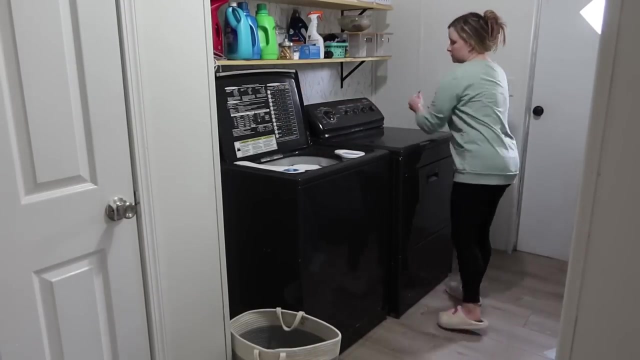 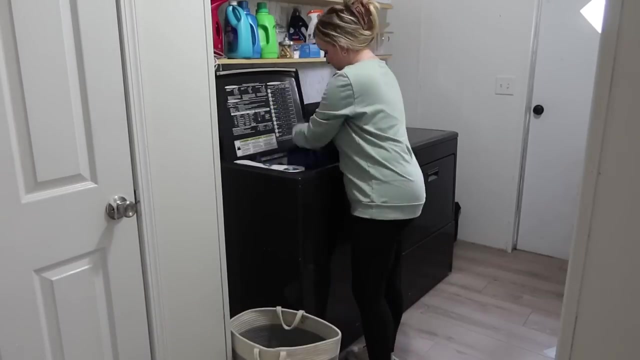 I know my mom taught me that I figured why we fool around so little and we keep track of time, being so serious idiots thinking it won't matter. keep me company downtown before the clock runs out. sun is shining, but the rain is welcome too. friends and nearby don't need another view. time is not on my mind, but then it's you. oh, I love it when. 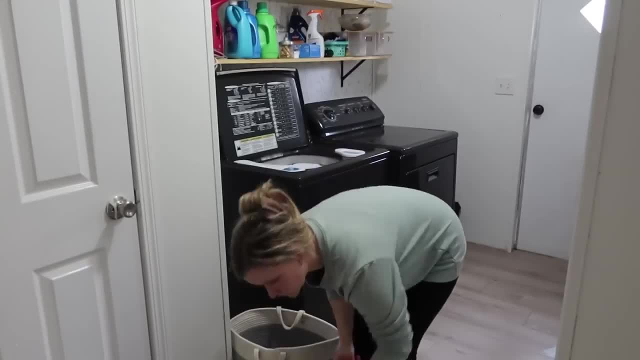 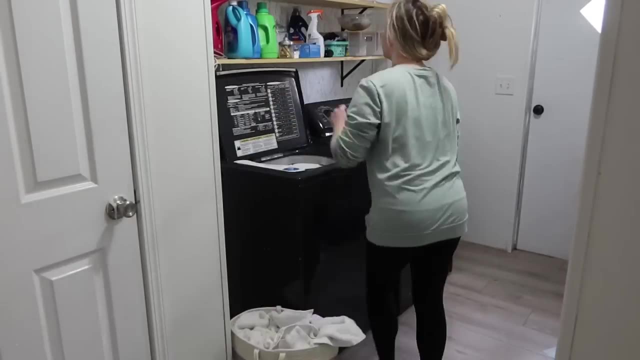 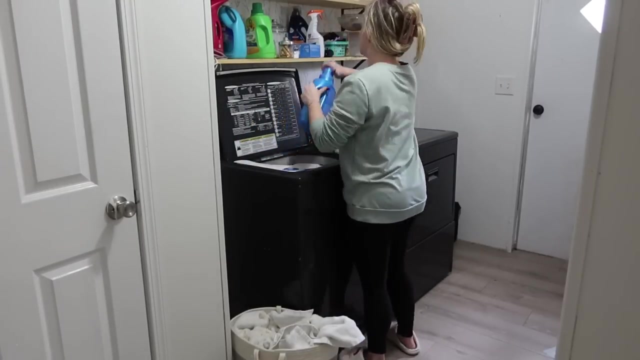 the love comes around, and then I remember all things must pass, but I'm not gonna wake up. wake up, I'm not ready. let me have another day. don't wake up. wake up, keep it steady, cause I'm happy. I'm not gonna wake up. no, no, not yet. 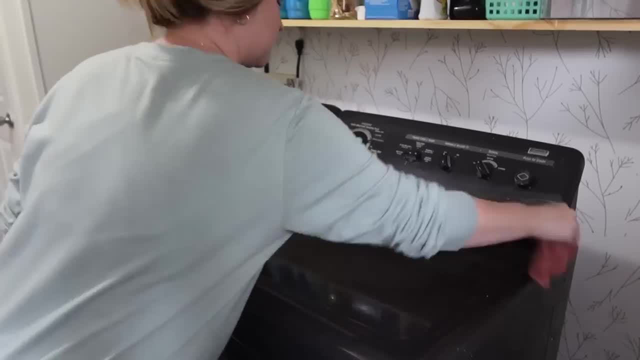 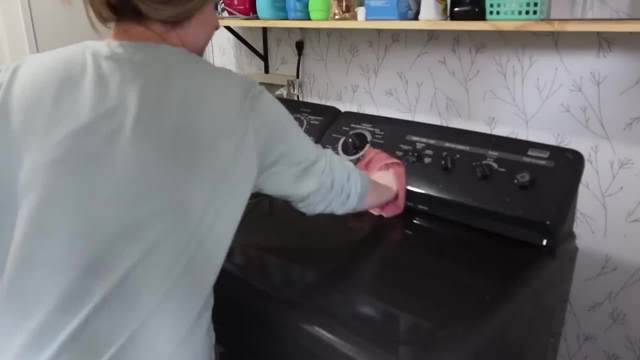 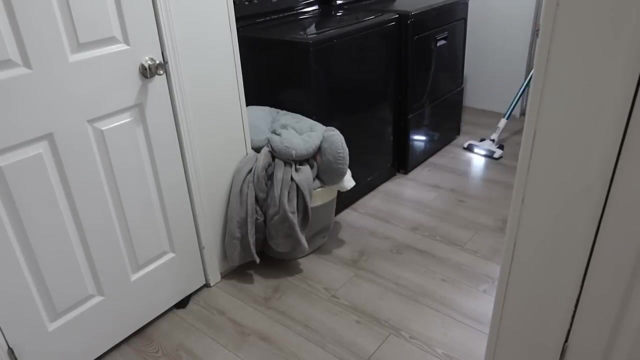 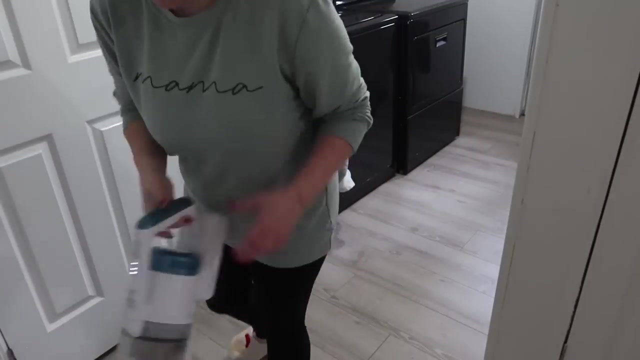 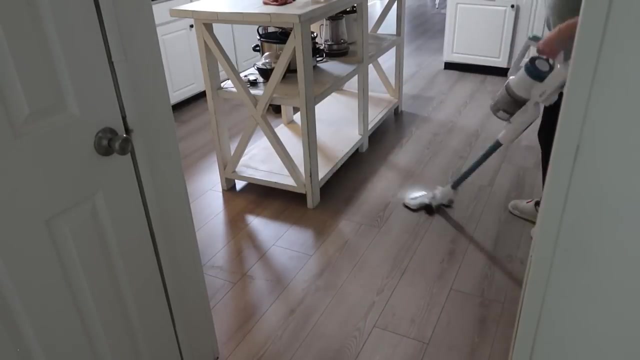 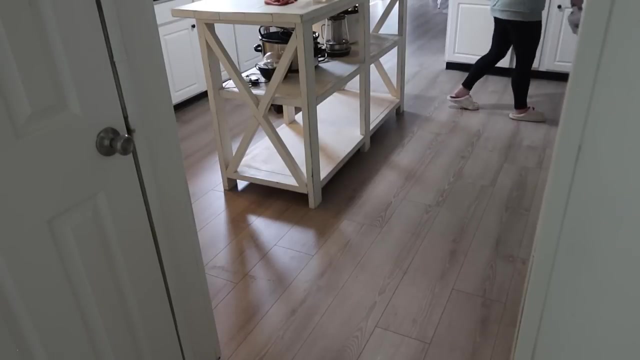 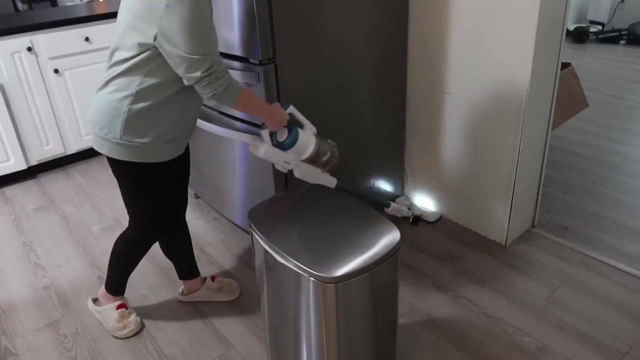 whoa, I'm afraid I'll end up nowhere. they keep saying I'll be fine. but how you know that I'll be there when it feels like I'm lying. every time someone asks how it goes and I save the details that actually mean something. you know that I mean when it happens. 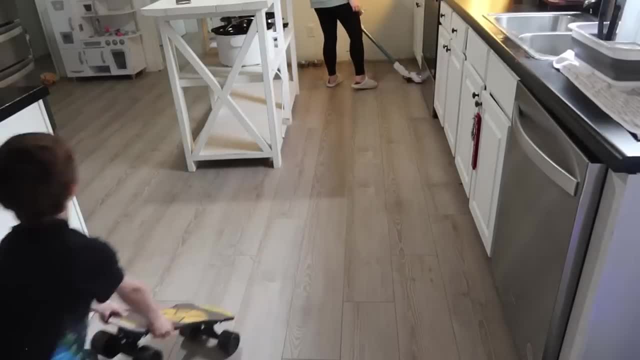 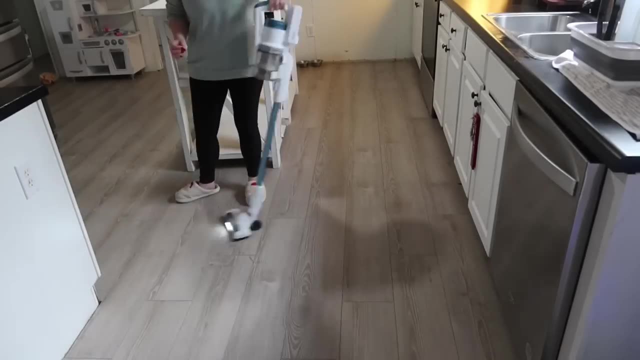 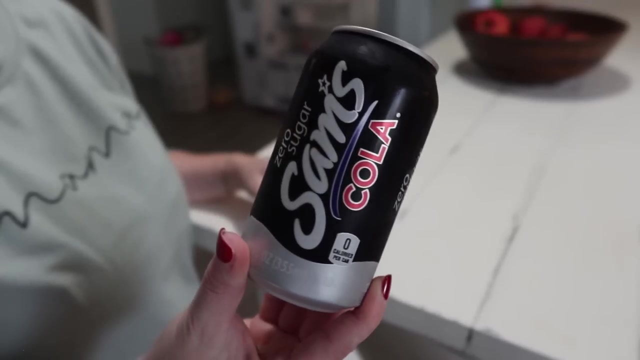 so now you can see it from a distance. you can, goodness, don't leave it to anyone alone. you only live for the moment. perfect, true? hey, we'll do it together. we'll do it one side at a time. be cool, ill, Limited. i had to take a quick, quick break. you guys and i was feeling a little hungry, but i didn't want. 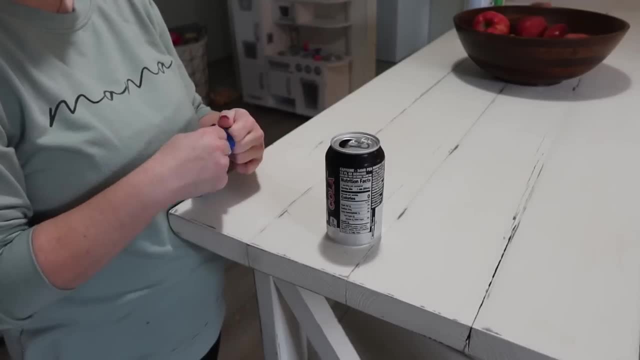 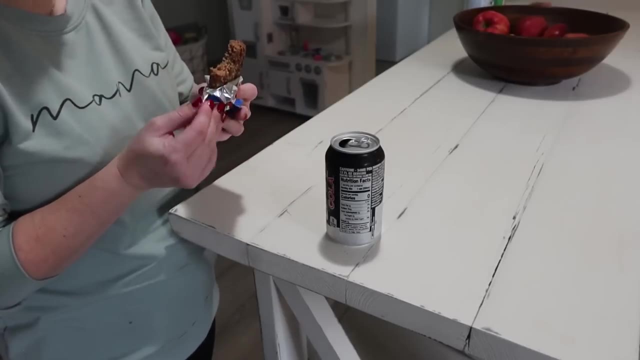 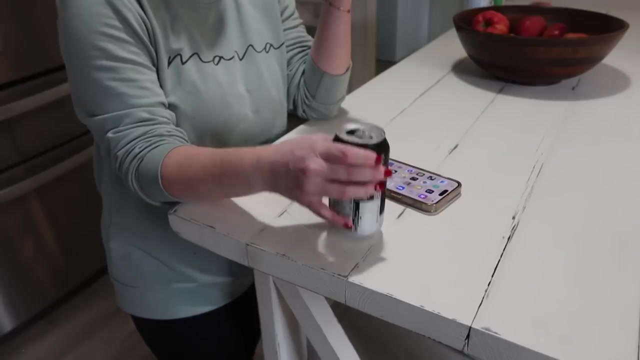 to eat a lot, because i knew if i ate like an actual lunch, then i was gonna feel tired and want to go to bed. so i'm just having a cliff bar and sam's cola zero scrolling on facebook and we're gonna get back at it. i only had the living room and the dining room left, but honestly, 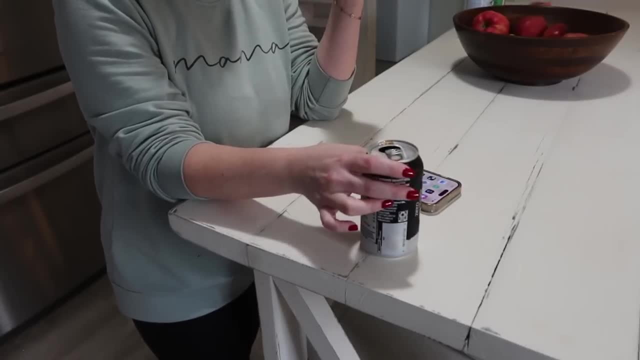 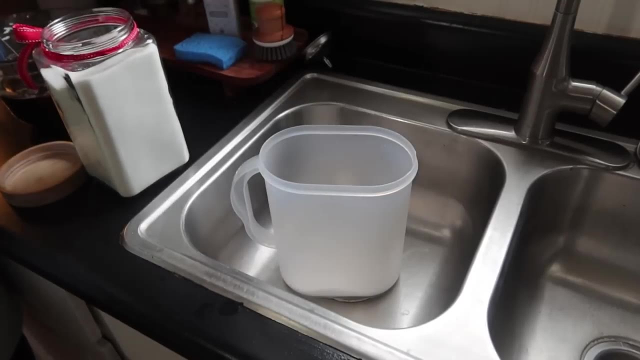 the living room is the worst out of everything, as you guys already saw, so i had to stop and take a breather before i jumped into that. it's like every time i walk into that room i feel so overwhelmed, but once i got it done, it felt so nice really quick. i'm gonna get this tea. 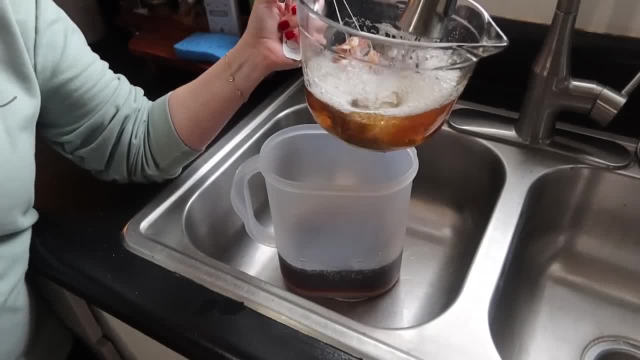 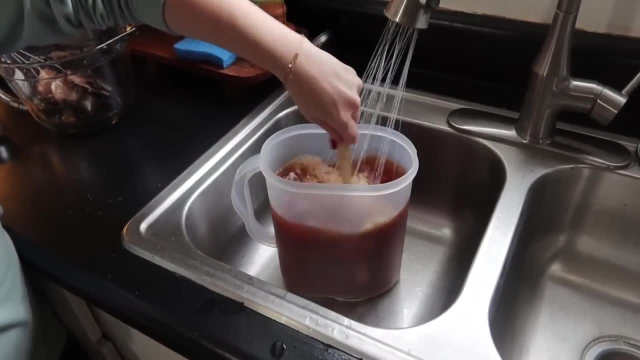 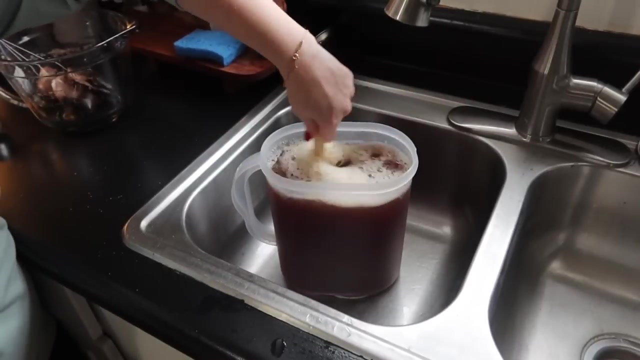 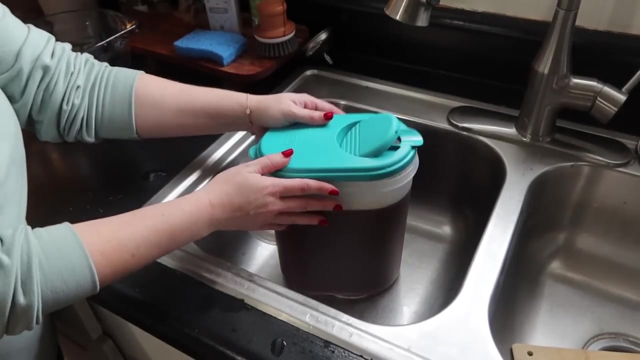 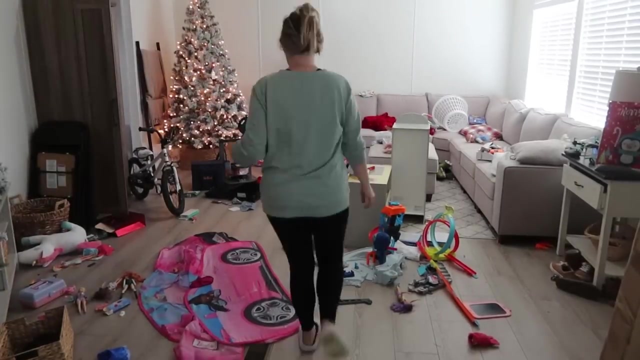 mixed up and we will go ahead and head into the living room. i'll be losing what to do. could somebody come and take me away? i've been in the tea without you and i got it in my head night and day, getting started um, jumping in by going ahead and removing the bigger stuff first they got. 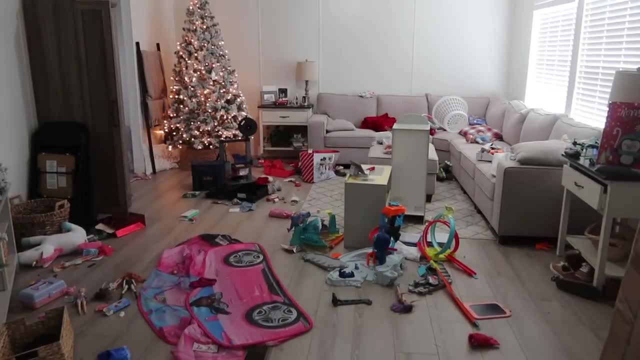 bicycles for christmas and also a little grocery store that i ended up getting for them. some of this stuff is a mix of stuff they got christmas morning and stuff that they got from our family members houses. everything just kind of got put here in the living room. so 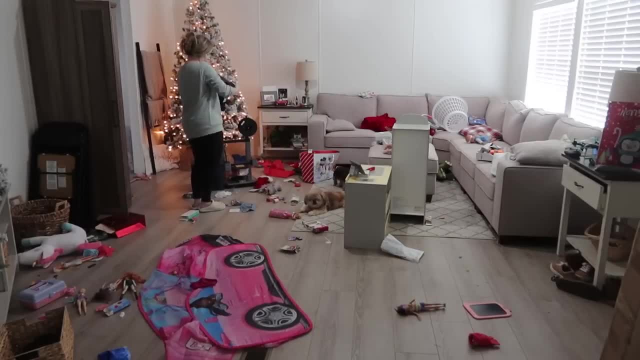 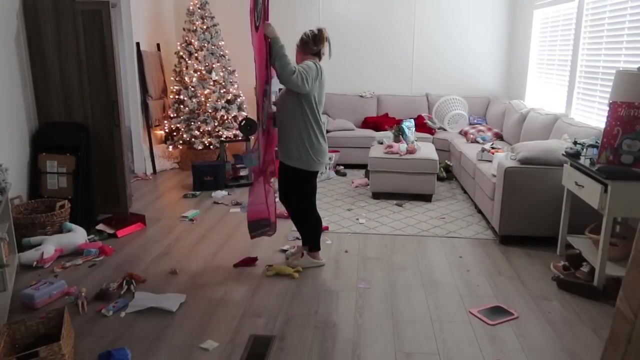 once i got that bigger stuff out, it wasn't as bad. i had a lot of like little stuff on the floor too, a lot of trash, and ray got some barbies for christmas and she has tons of little barbie accessories everywhere, and so what i did is i eventually grabbed the laundry basket. that's on. 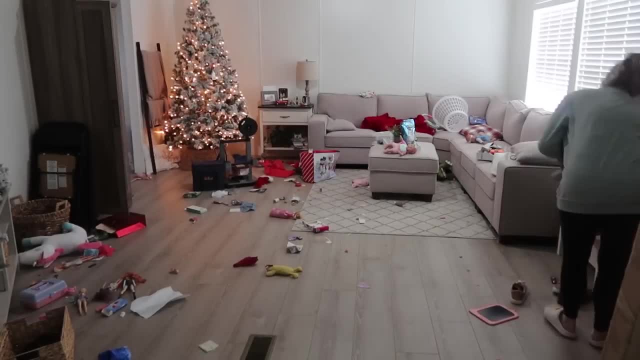 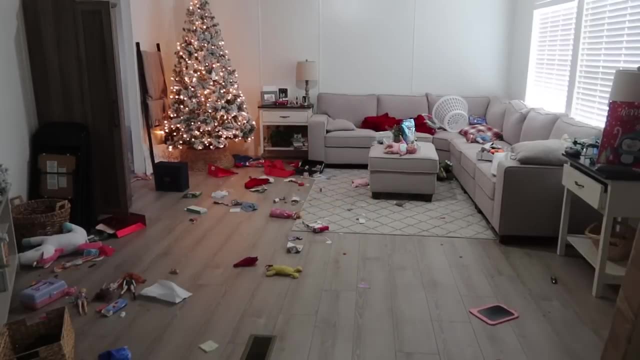 the couch and i just started throwing all the toys that needed to go to their rooms into the basket and once i get it in the room later i'll get it sorted and everything. a little later on in the video i do get her barbies organized somewhat under her bed. it's not exactly the way that i want. 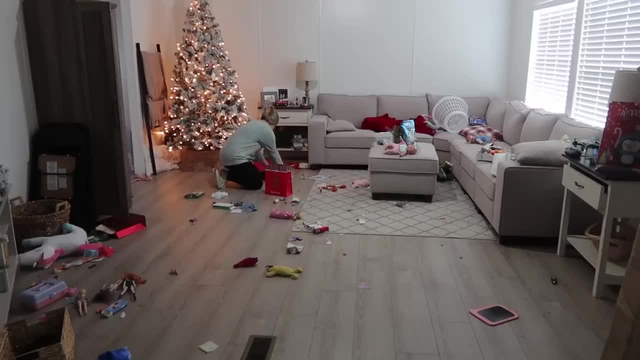 it, but it's a way that's going to work for now. she got so many barbies for christmas, i think everywhere we went she got a barbie and they all have those little tiny accessories, so we had those everywhere. same with kane. he got lots of hot wheels. he is into hot wheels this year and so 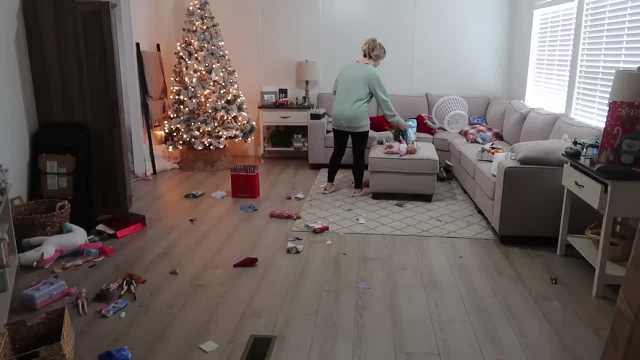 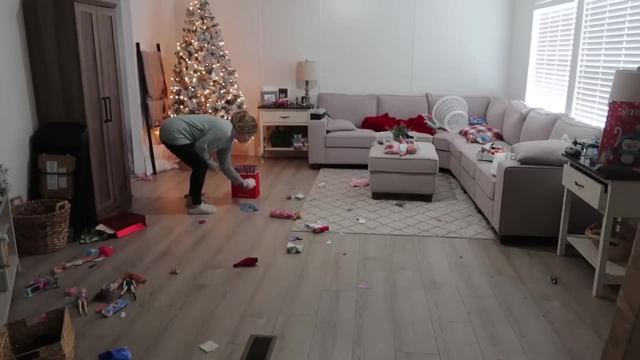 what he got, and he got tons of them. hi, bless him, he has gotten a lot of stuff for his room for christmas, and so he has been in his room cleaning it non-stop, and he's been decorating and setting his stuff up the way that he wants it. maybe in a future video i can show you guys how he's got it. 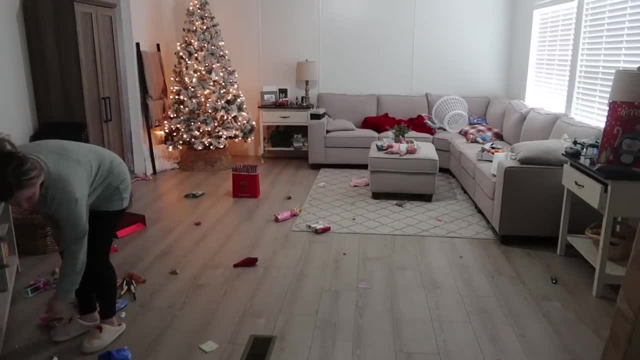 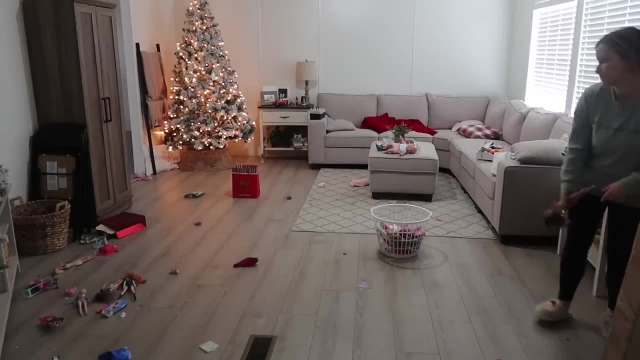 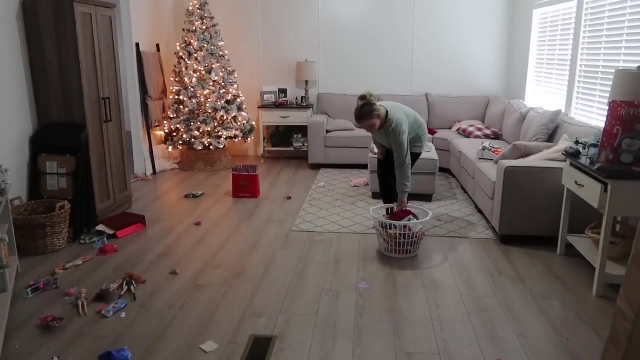 i'm kind of jealous at how he's got it, to be honest, because it looks so cool in there. he's got those little led strips and he got a lamp for christmas. honestly, he doesn't even need his regular light switch in his room anymore because of all the cool lights he's got in there. but, yeah, he is loving his room. uh, he also got some. 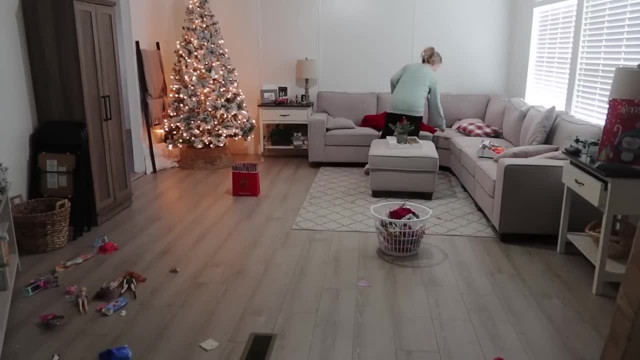 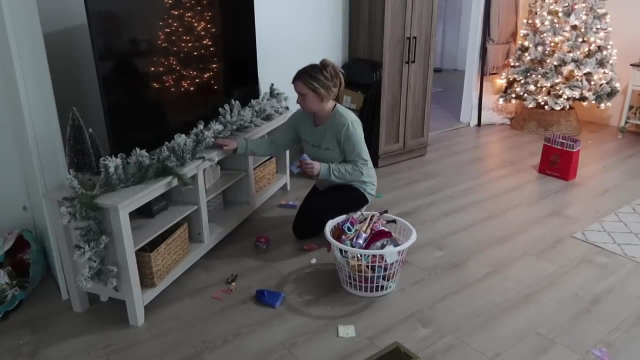 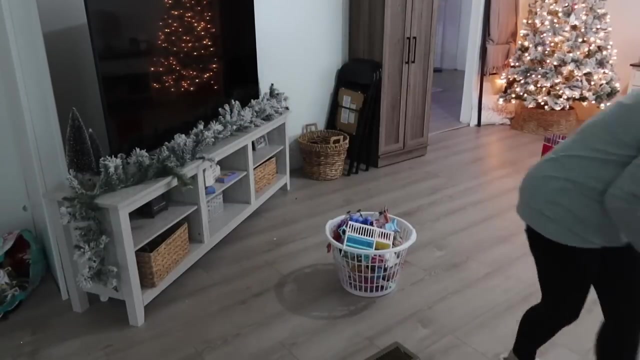 shelves for christmas, so he's been hanging those up and getting his robots on display. stuff like that just makes my heart so happy. he has waited so long to have a bedroom of his own and he finally has it, so just watching him decorate it the way that he wants it just makes my heart so happy. 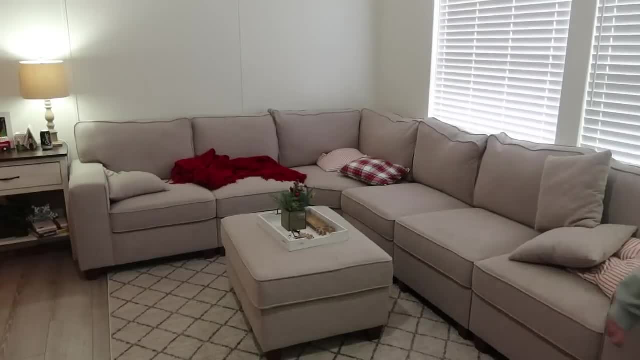 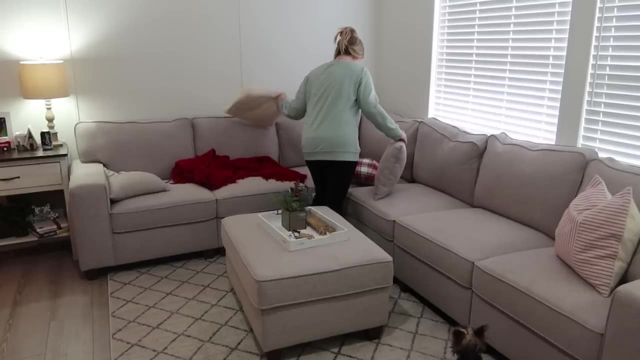 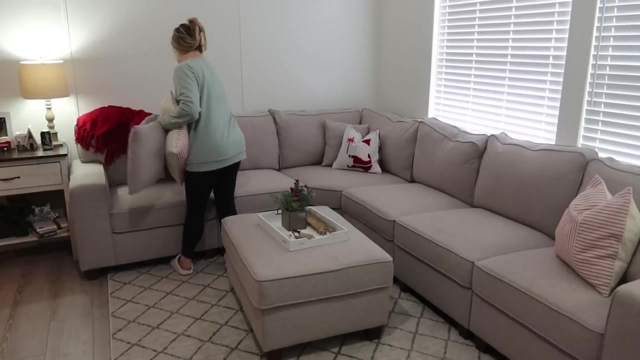 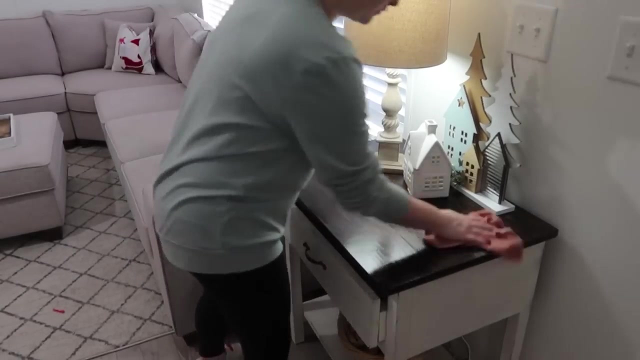 so here pretty soon i'm gonna be rearranging my living room. i should have that video out. hopefully next week that video will be going out. don't want to upload on new year's day because i know a lot of you will probably be spending time with your family. 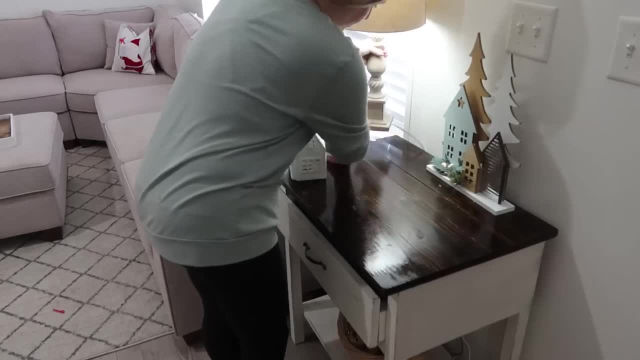 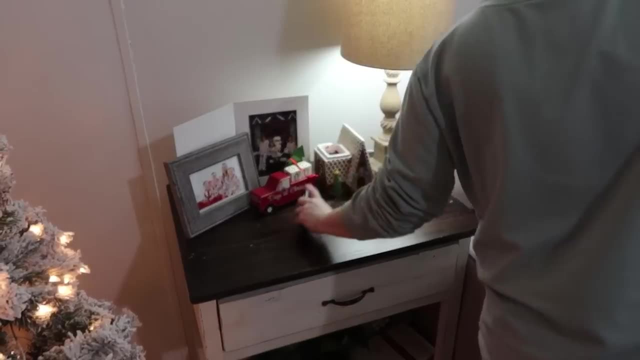 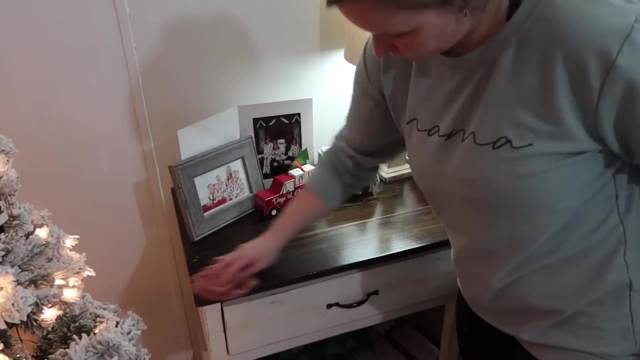 so it'll probably be after the new year that i'll upload it, but i'm so excited we're gonna be turning the couch around. the back of it is running with the front door and i'm gonna put my tv on the far wall where my christmas tree is at, and i've got a really pretty entryway table coming. 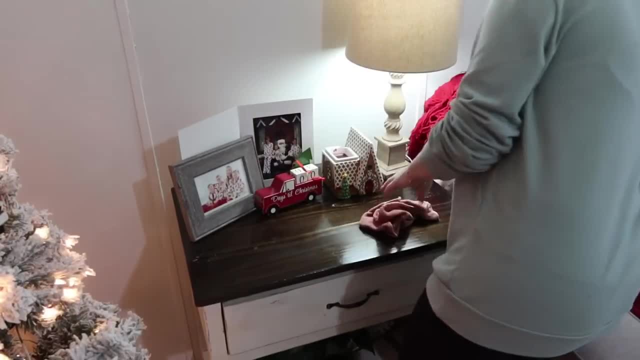 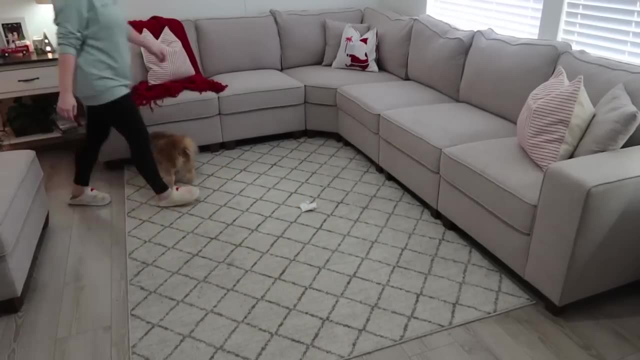 that i'm gonna put on the wall that the tv is currently on. there's just a whole new setup that's gonna be happening and i'm gonna be putting it on the wall that the tv is currently on and i cannot wait to get it all together. so make sure you guys come back for that video to see how. 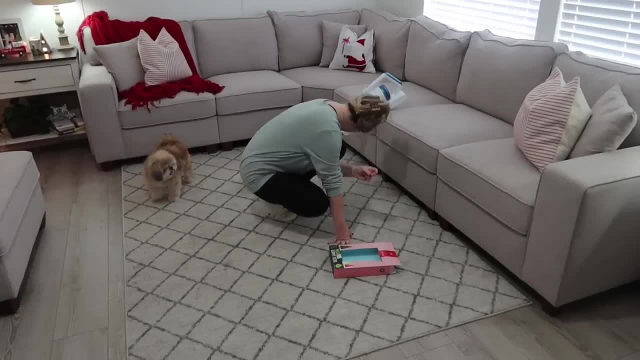 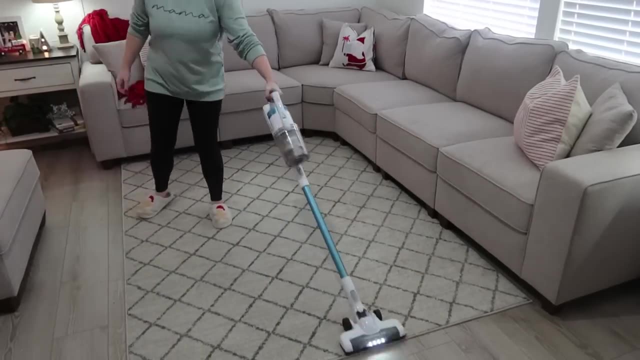 it all turns out, but with that setup i don't know if i'm gonna be able to keep my christmas tree up or not. i'm hoping i can stick it over in the corner or maybe even leave it where it's at, who knows. but i'm just so excited to finally get my living room rearranged the way that i want it, and 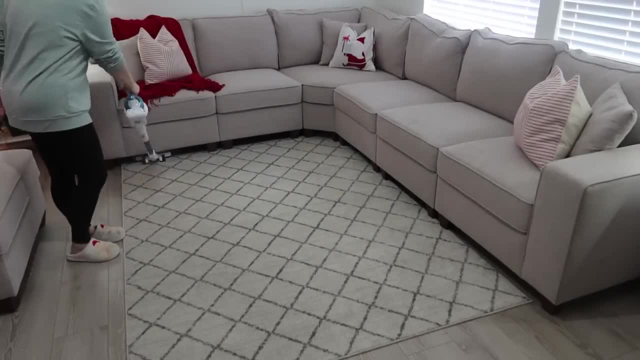 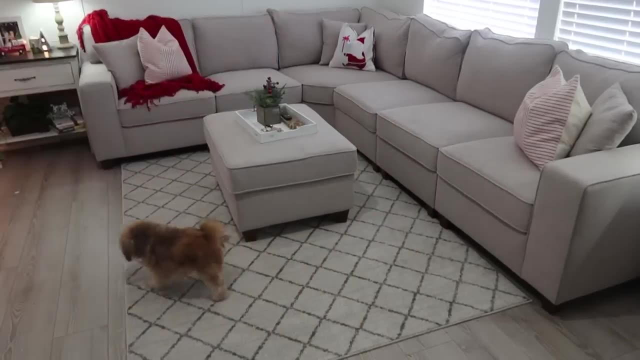 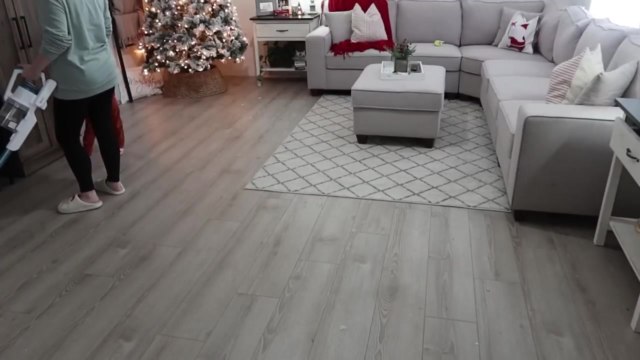 later in the month we're gonna be working on my laundry room. i'm gonna be adding a coat nook in. i'm gonna do some organizing. i got some rugs to go in there as well, but i've got this whole idea going for the nook. by my back door. there's a little nook in the wall and i think it's gonna 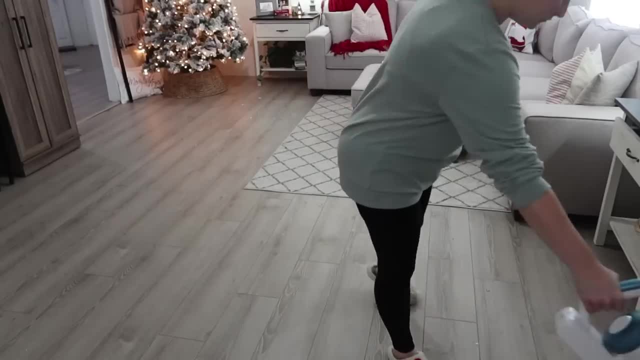 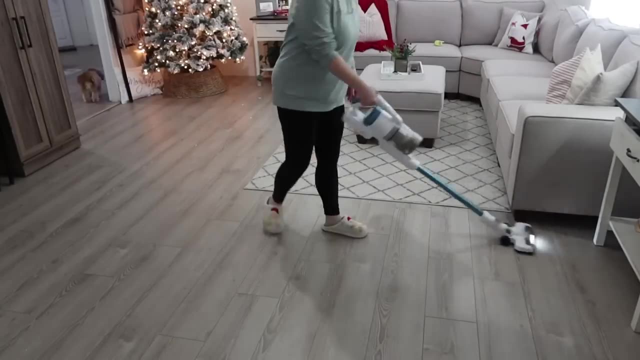 be perfect for a place to put coats. so i'm gonna hang some boards on the wall. we're gonna paint it, um, hoping i can do some kind of shoe organization as well, but i think it's gonna look really good. so that'll be happening later in the month. 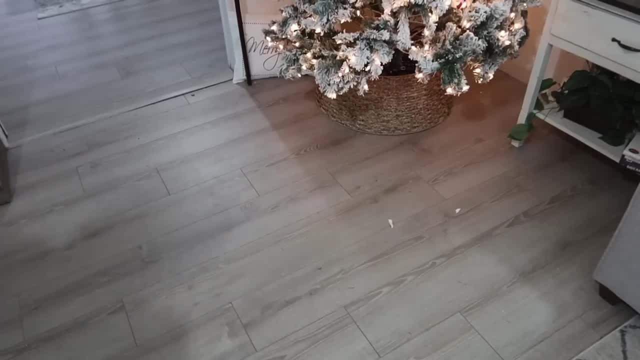 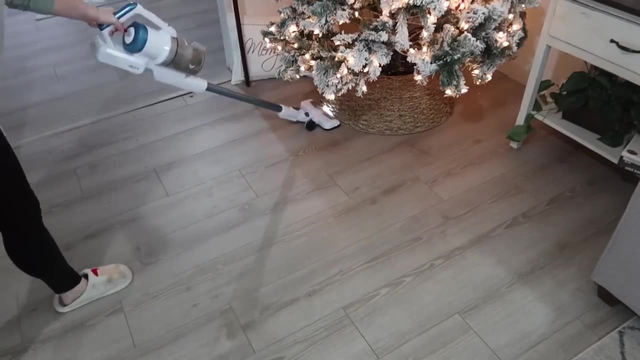 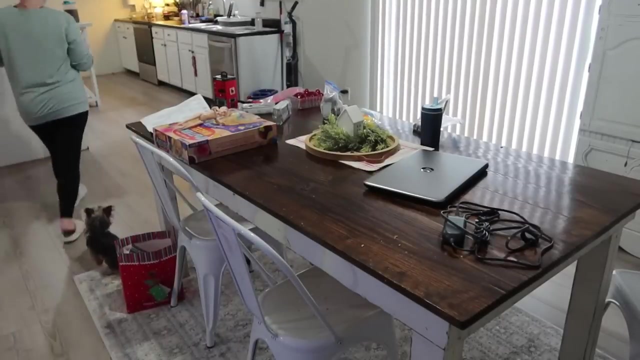 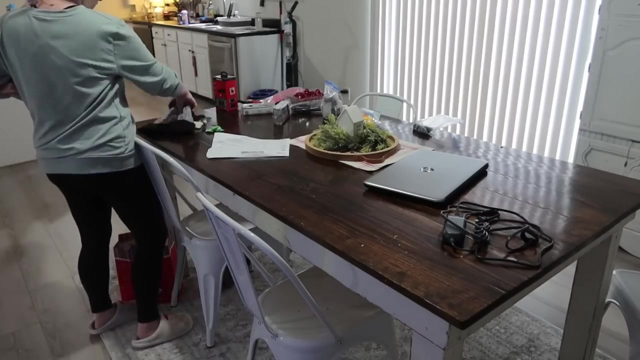 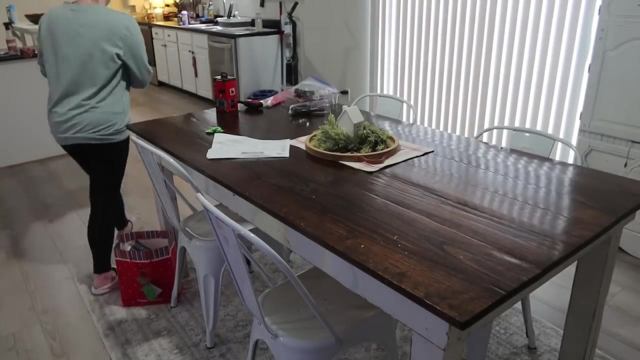 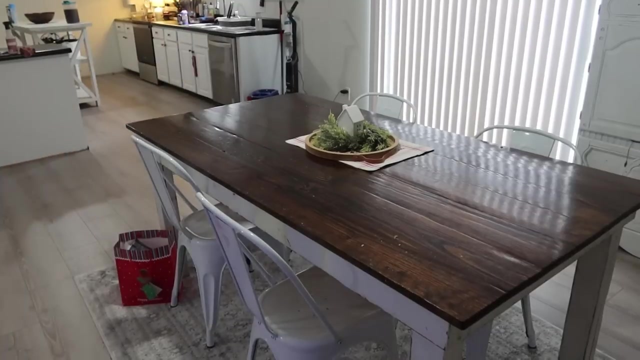 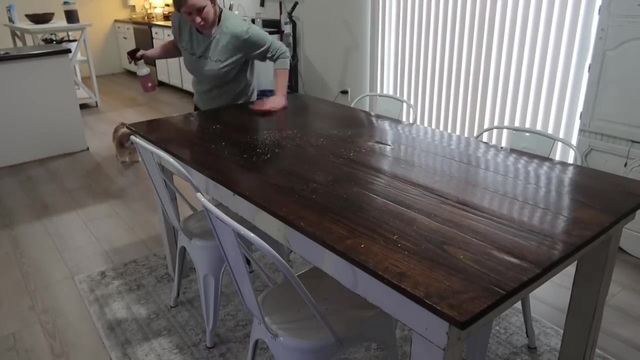 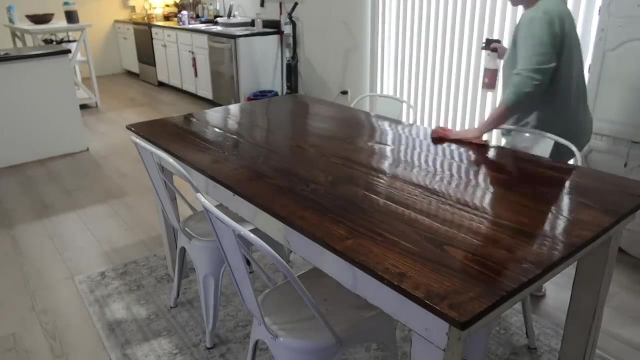 you're smiling, that's for sure funny how you had the best of. i don't know if i make it home. i don't know, only know i want the best of us, so i'll be the last to stay. pretend i don't know how this night will end. 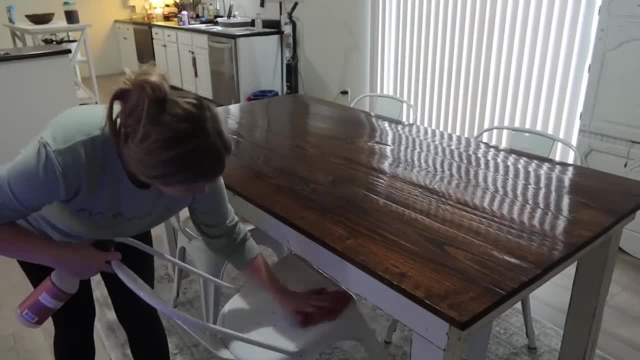 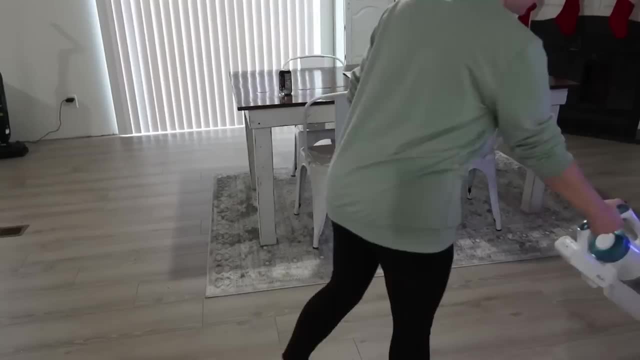 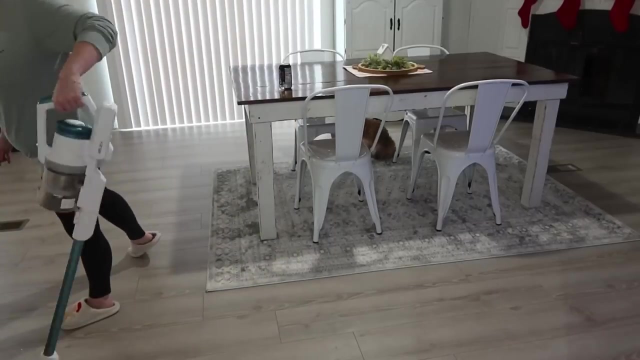 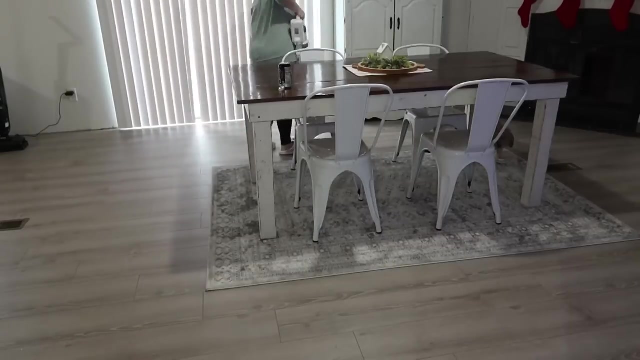 i'll be your heartbeat. the dj plays. oops, i did it again. i don't know if i make it home. i don't know, not like i can. all i know is that this only know. i want the best of us. so when nobody's away, i'll be the last to stay. 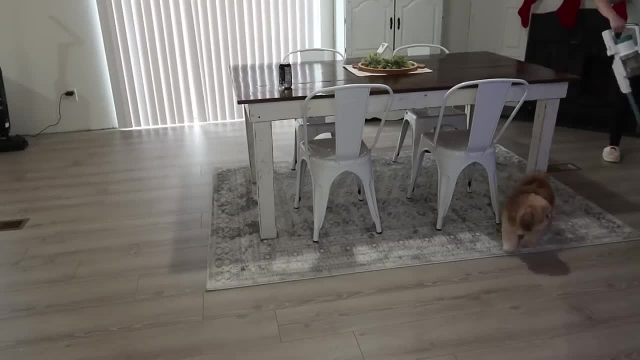 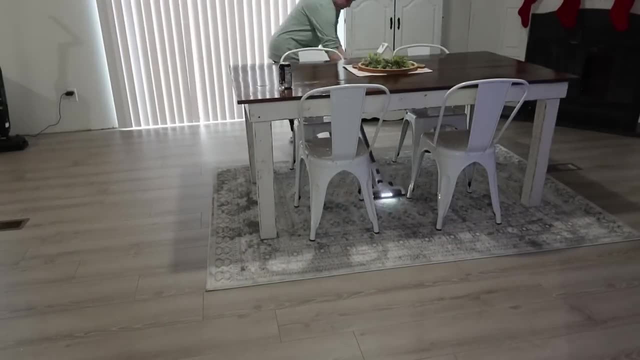 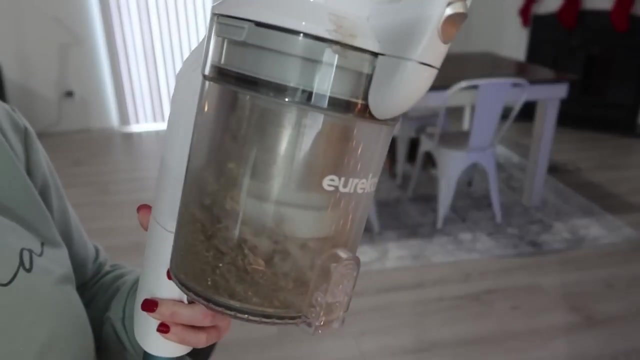 i'll be the last to stay, and i there's the night away. no matter what they say, i'll be the last to stay and i there's me night away, when nobody's awake. i'll be the last to stay and i there's the night away. 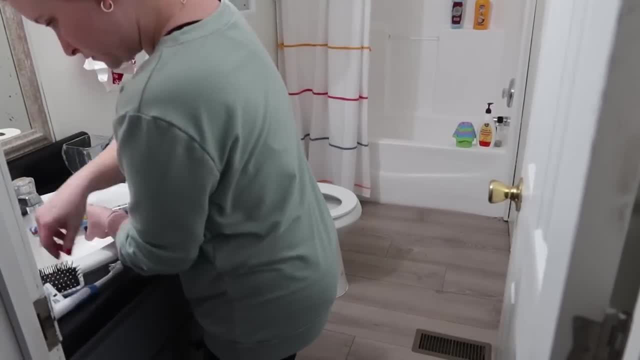 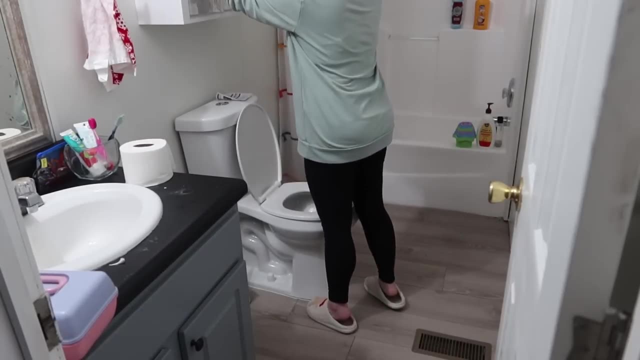 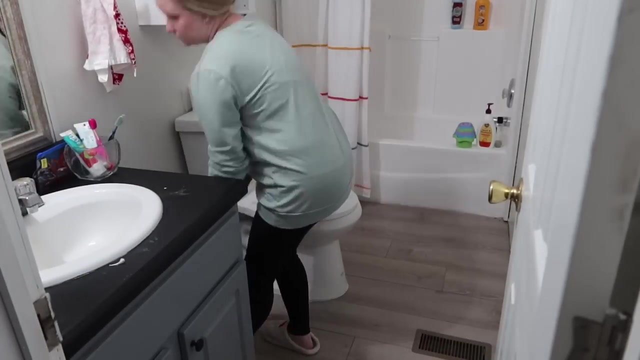 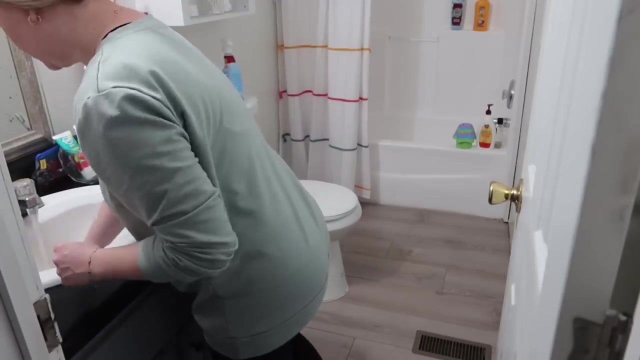 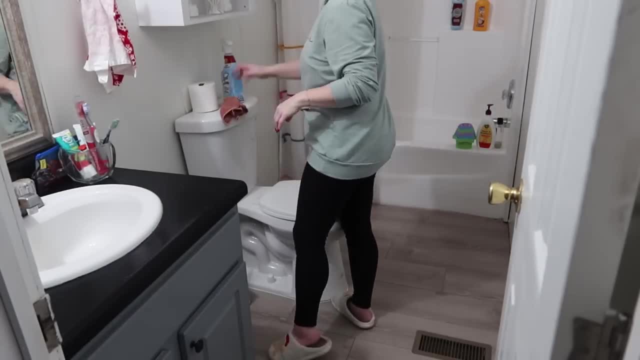 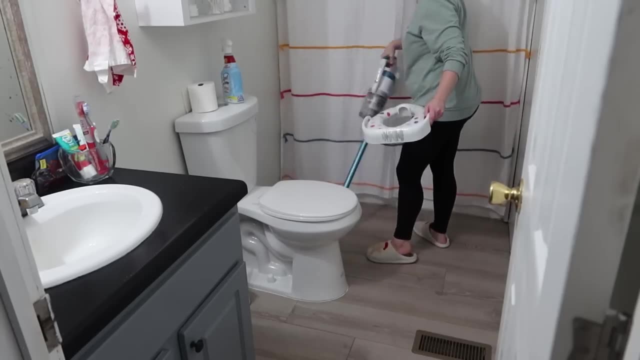 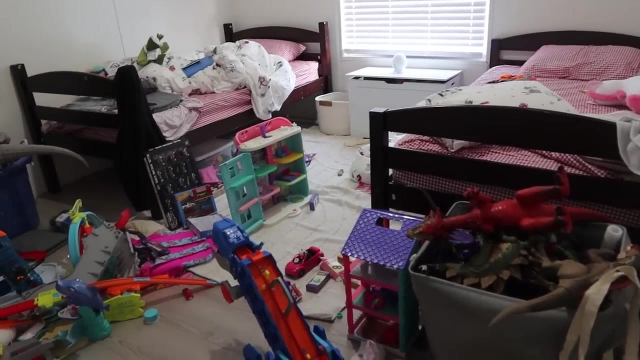 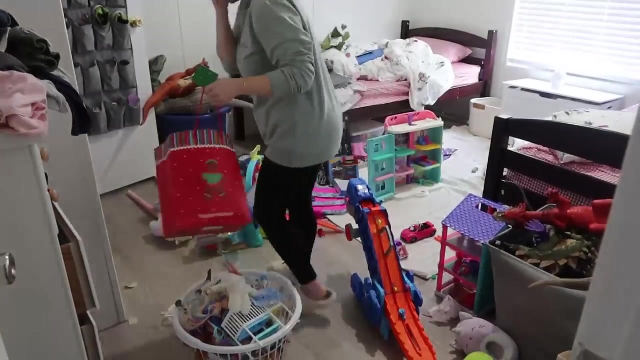 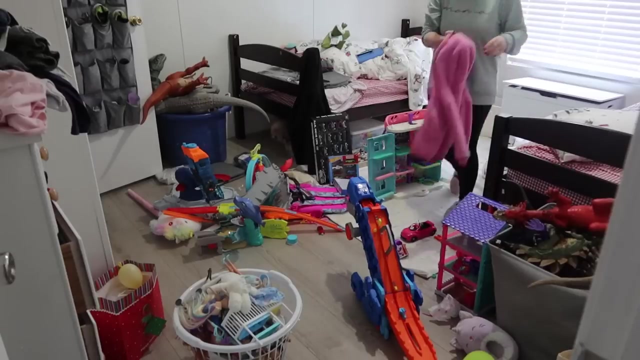 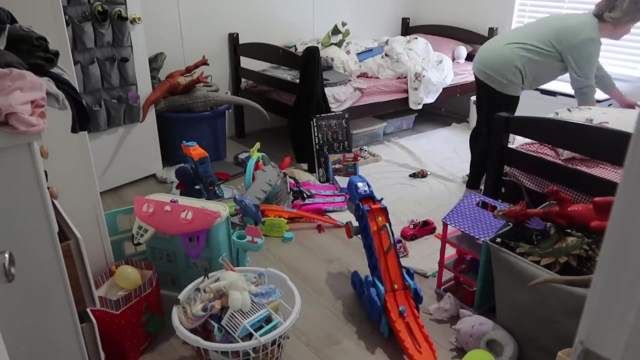 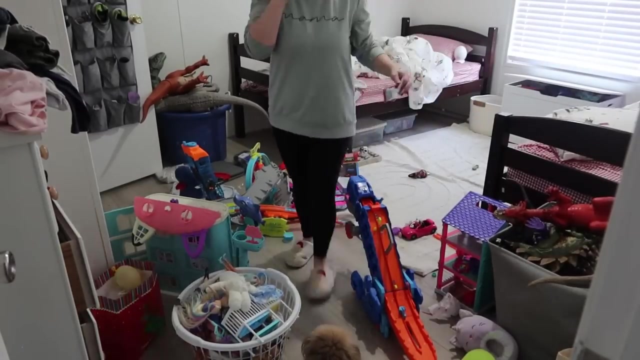 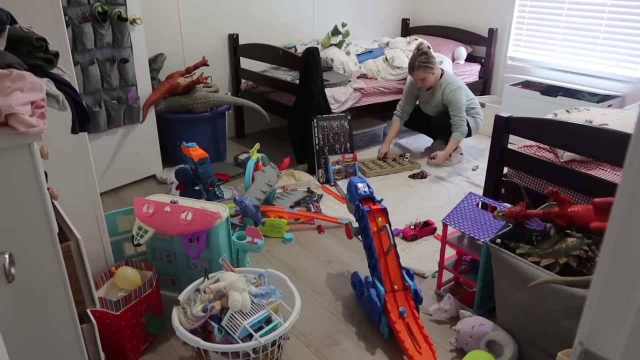 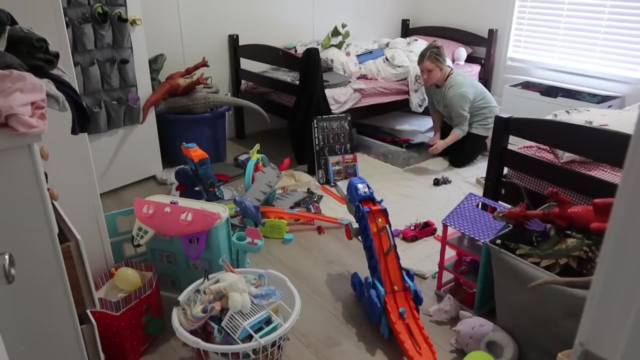 That's the night away. when nobody's awake, I'll be the last to stay. That's the night away, no matter what they say. That's the night away, no matter what they say, That I've got under his bed. This container works perfect for his Hot Wheels. 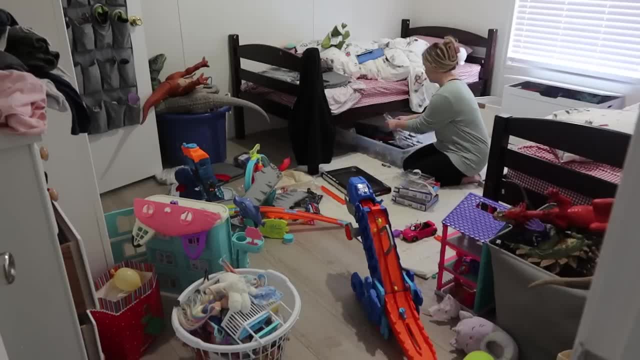 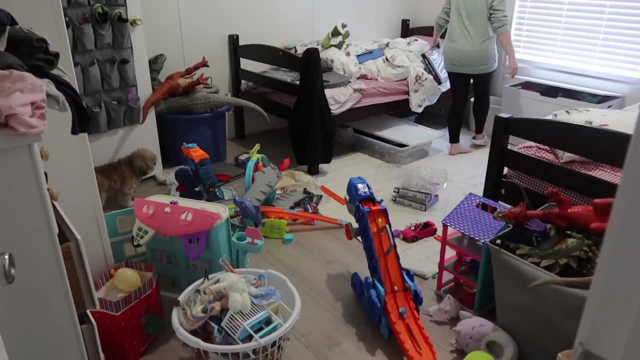 It holds all of the cars Which Santa did bring him a case for Christmas So he can put some of the cars in that. But this container works perfect for all of the tracks and stuff When he takes his tracks apart- Some of his tracks he had put together. 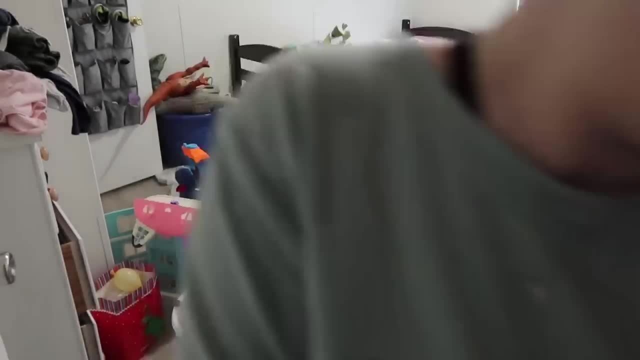 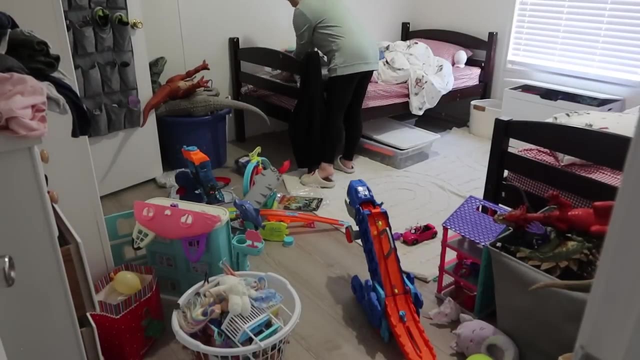 So I'm not going to be taking those apart, Because he worked really hard to get them built. So I'll just stick those over in the corner. But everything else I'll go ahead and put into. That's the night away, no matter what they say. This container here under his bed. 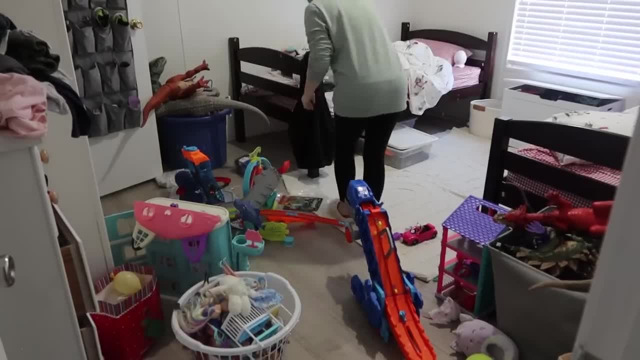 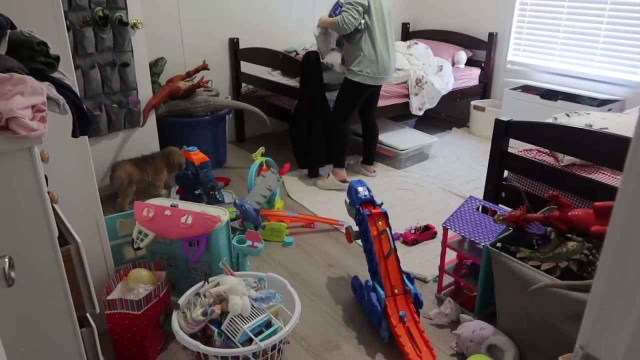 I want to get one for Ray's Barbies. I think that'll work perfect to hold all of her Barbies And her accessories. But I didn't have an extra one, So I ended up pulling a couple of plastic containers That I already had that I wasn't using for anything. 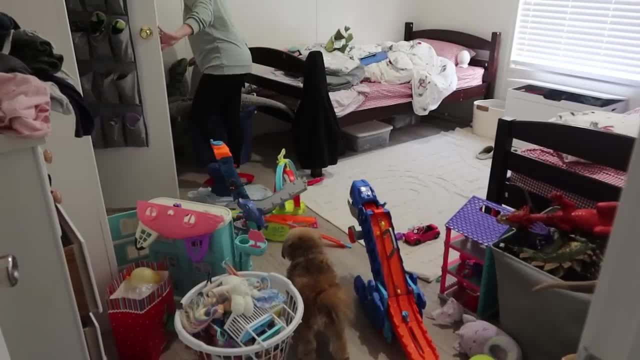 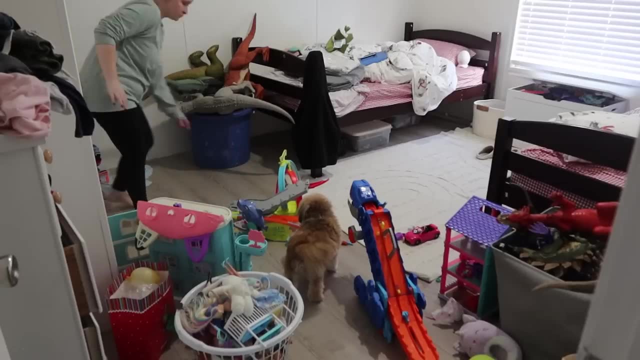 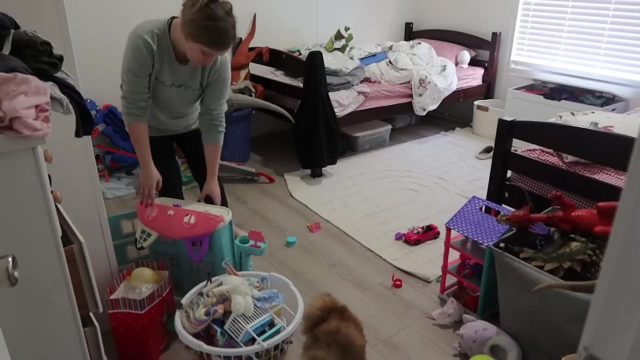 I used for her Barbies and accessories for now, And I'll put those under her bed, As well as both of the dollhouses. I also hang this on my bed And I've been using this for six months now. I bought this for my daughter. It's like an hourglass. 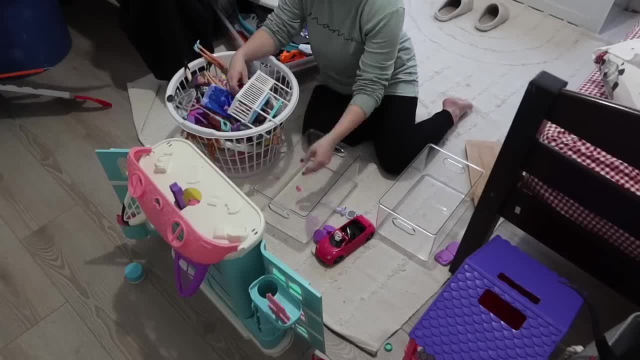 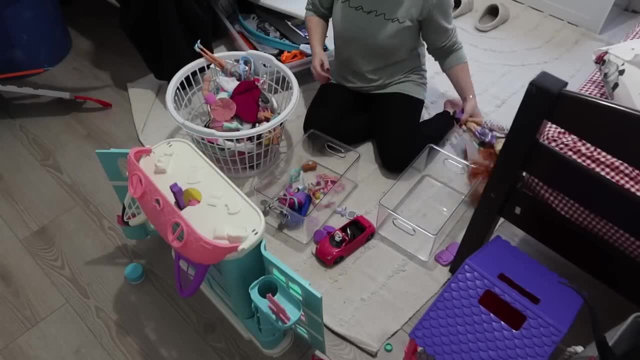 And she loves it. I have a book, I have a book, And here's the book. And then here's the page. I have my littleangers. No one's gonna read them, And I'm not kidding. I've been using this for 12 years And I've been taking them out. 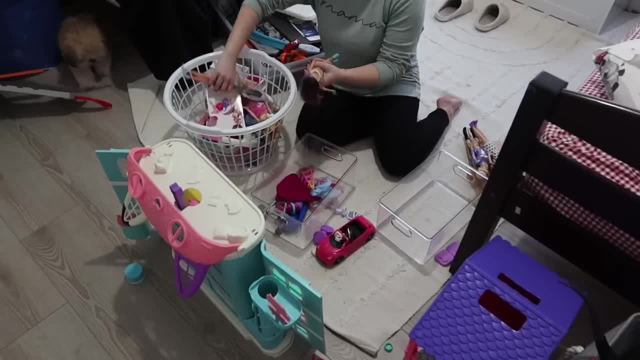 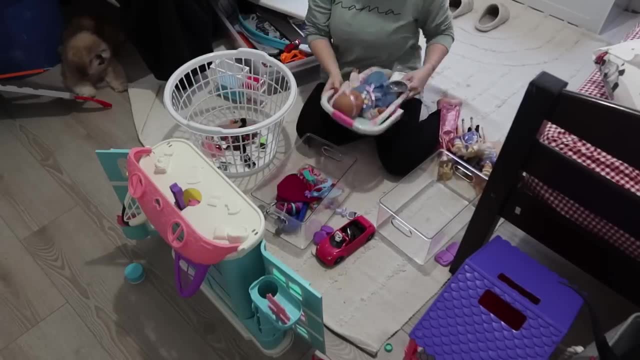 If they're crazy to come and visit, I'm going to eat them. We're going to take them out. They're going to take them out. I'm going to take them out And I'm going to go put them in my bed. Remember it, I know. oh, oh right. 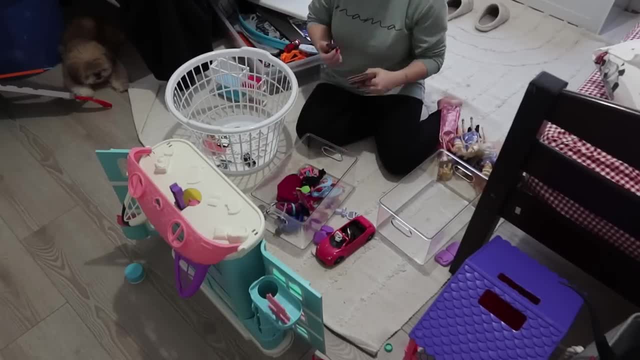 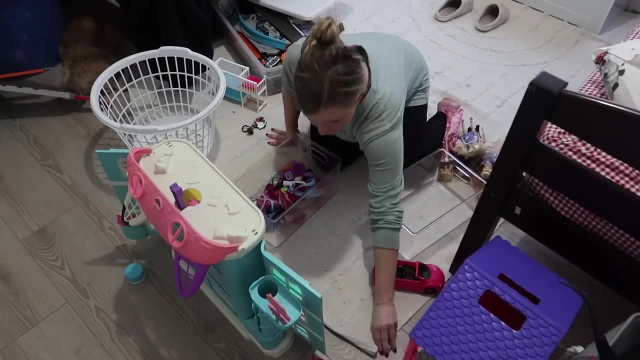 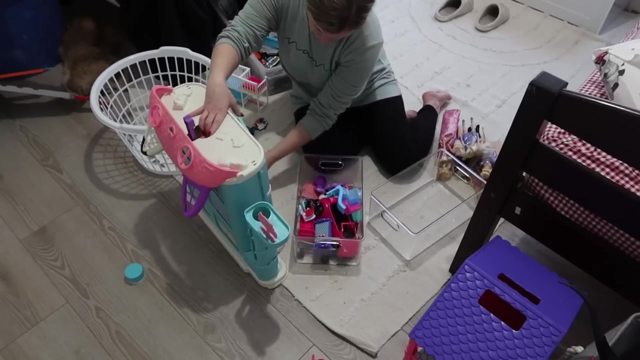 That these are just feelings. But these ones, they feel like they For just one reason: Slide on me, babe. slide on me, babe. I wanna make you feel good. Trap on me, babe. trap on me babe. Play a trick, I feel smooth. 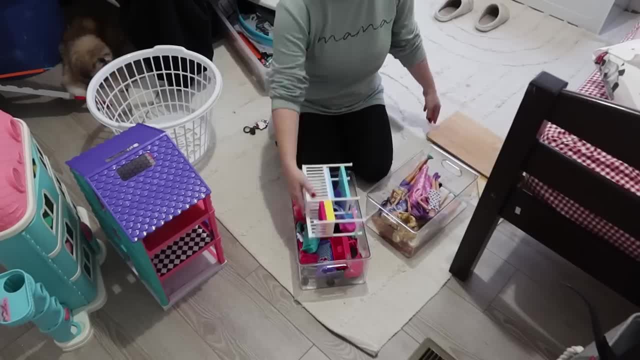 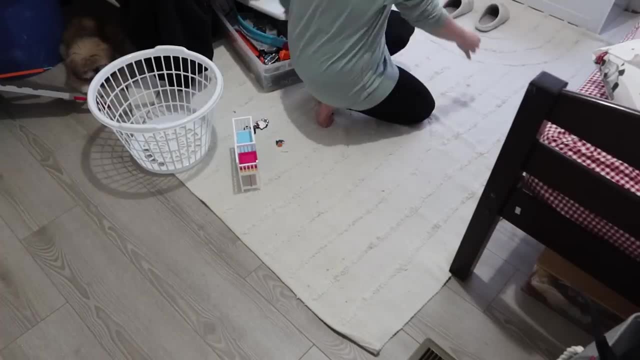 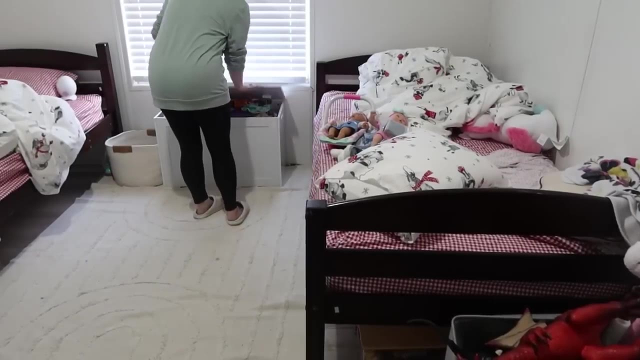 Slide on me, babe. slide on me, babe. I wanna make you feel real good. Trap on me, babe. trap on me, babe. Play a trick. I feel smooth. So we took a ride- One last part, with the best kind of sight, But I always found that we're out of time. 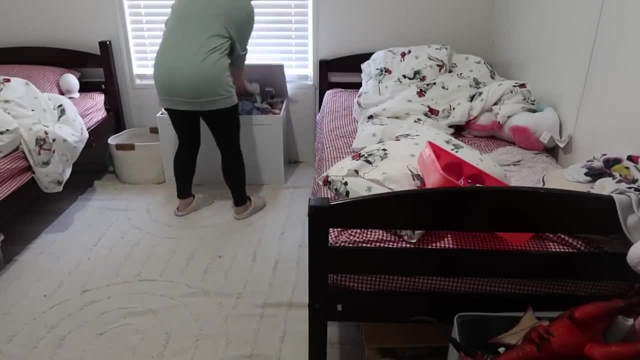 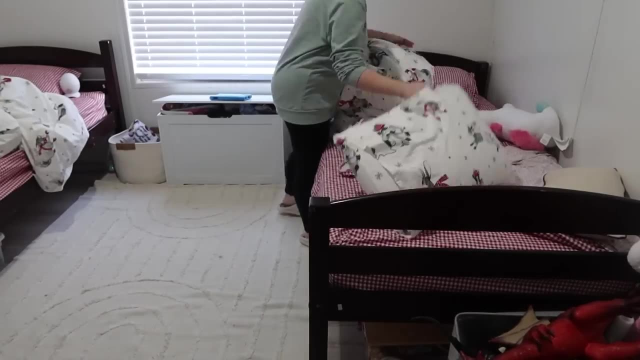 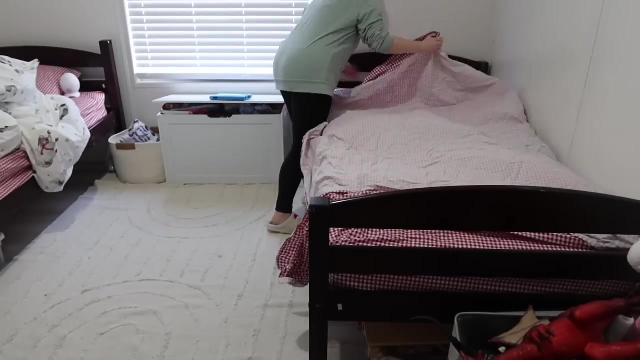 And this city made me realize. I know, oh, oh right, That these are just feelings, But these ones, they feel like they. They might not quite, But these are just feelings, But they feel like they For just one reason: Slide on me, babe. slide on me, babe. 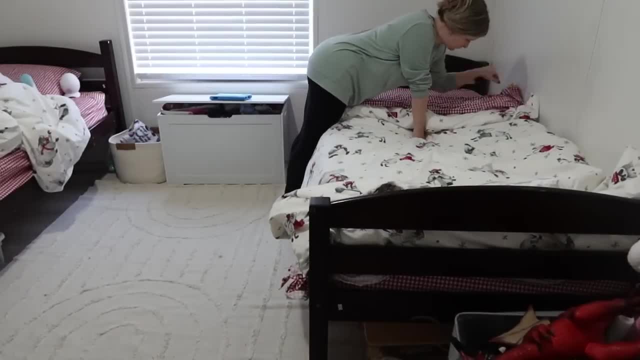 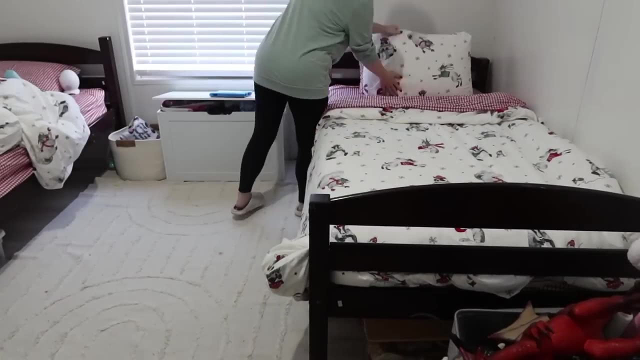 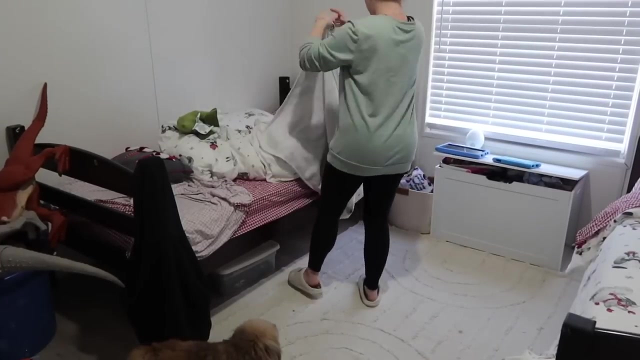 I wanna make you feel good. Trap on me, babe, trap on me babe. Play a trick, I feel smooth, Slide on me, babe, slide on me babe. I wanna make you feel real good. Trap on me, babe, trap on me babe. 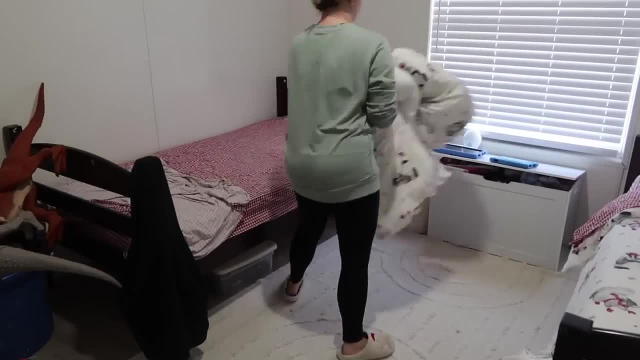 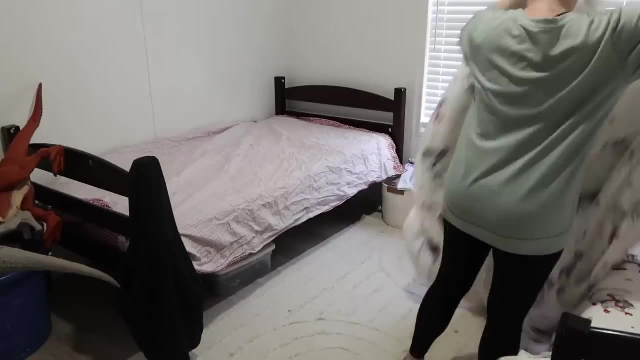 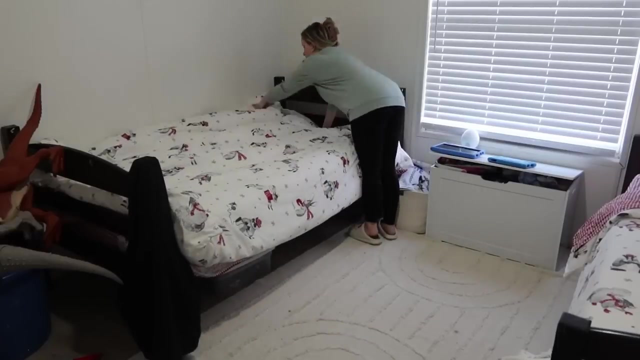 so i'm probably gonna leave their christmas bedding on for a little bit longer. i just don't want to take it off yet. it's really cute, but the good thing about these duvets is that i can just change the covers on them. so when that time comes, it'll be really easy, and i just like the idea of. 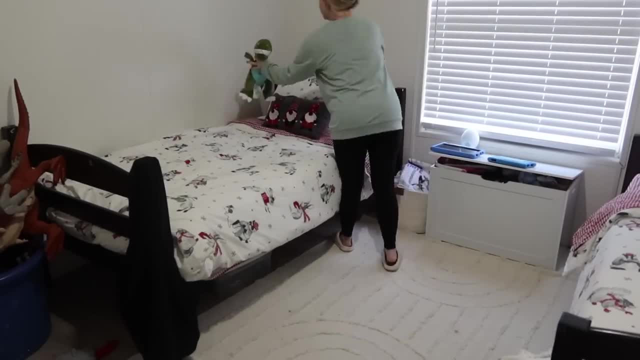 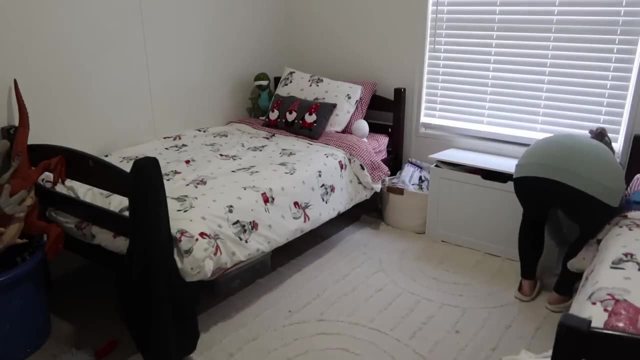 duvets, because you can easily switch them out without having to store comforters away. comforters take up so much room, and so i really like the idea of just you know, being able to replace the covers, and all you gotta do is store the covers away. my mom had got them some throws for christmas, so i'm